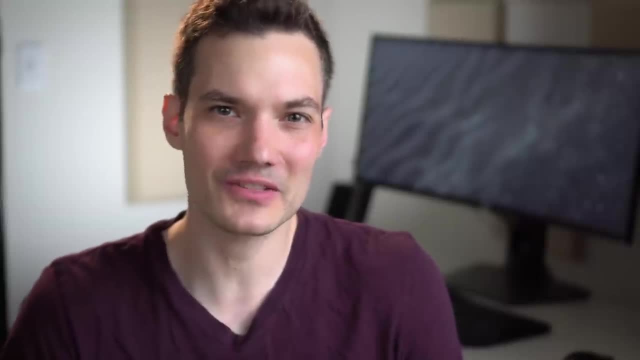 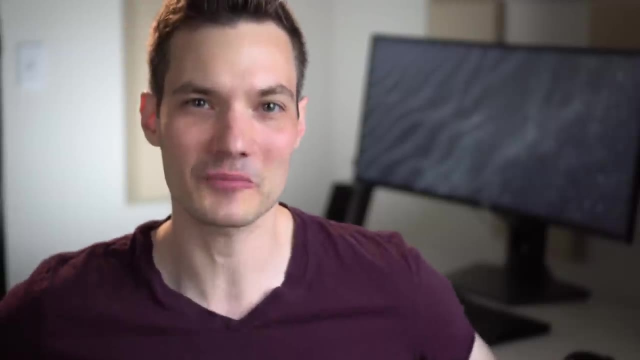 I could revert back to previous versions. I can compare the differences between different versions. I could see who changed what, Basically. if I screw something up, well, I could just jump back to a previous version, Now that we know what Git is next. 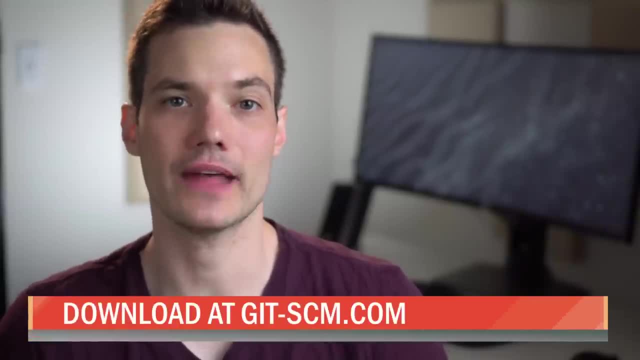 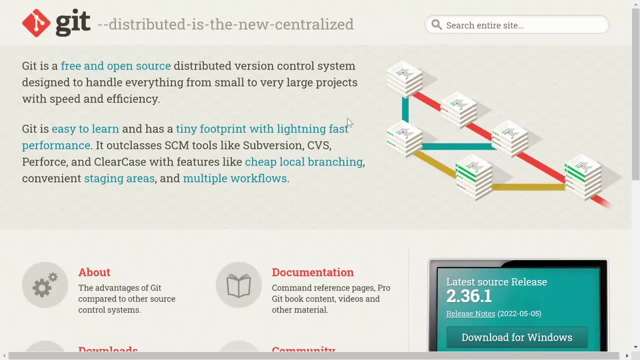 we need to install it on our computer, and to do that you can head to the website up above or you can click on the link down below in the description. Once you land on the website, click and then select your operating system and then run through the installation process. 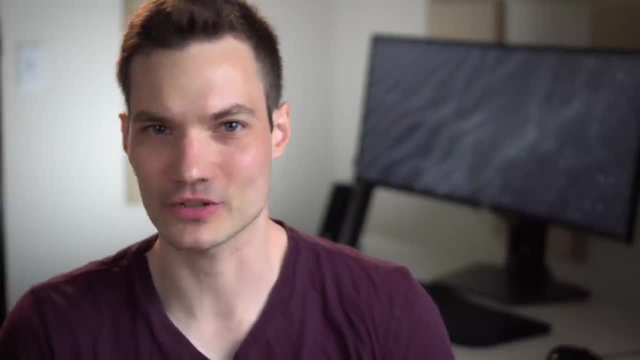 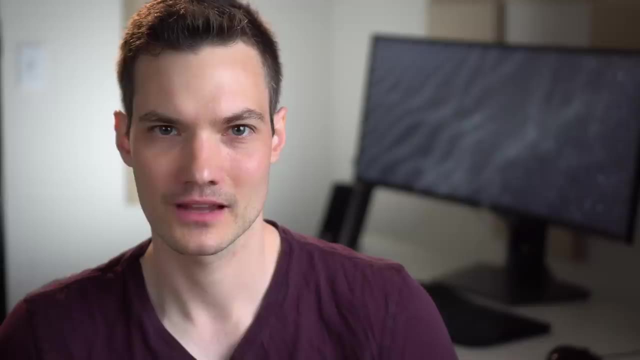 When I installed Git it came with a terminal called Git Bash. To launch it, simply click on your start menu and then type in Git Bash, and then you can launch it. but you could also use any other terminal that you have on your computer. 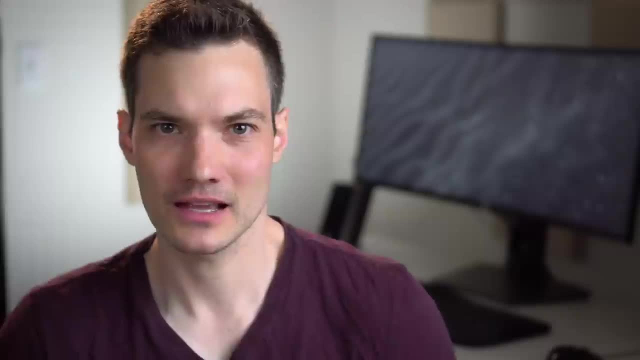 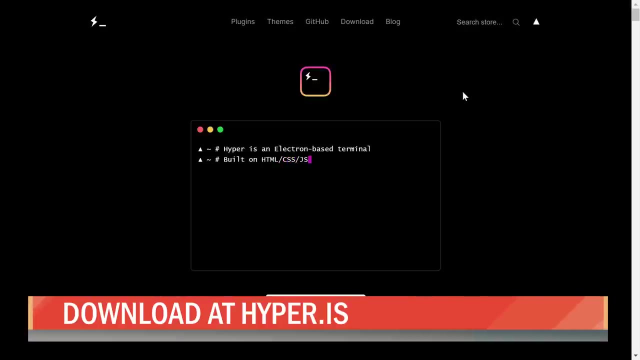 You could also use PowerShell or Command Prompt. If you're on Mac, you could use the terminal that comes with your machine. You could also download third-party terminals like ids, and that works across all different platforms, so the choice is really yours. 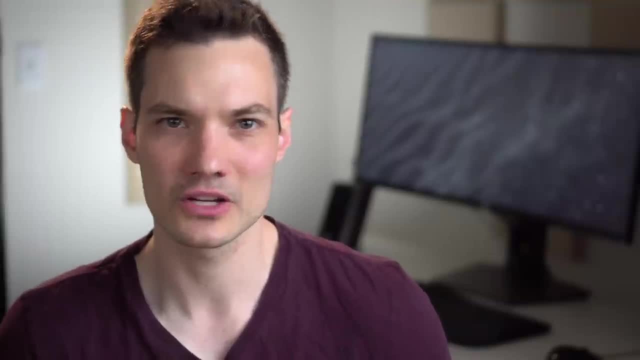 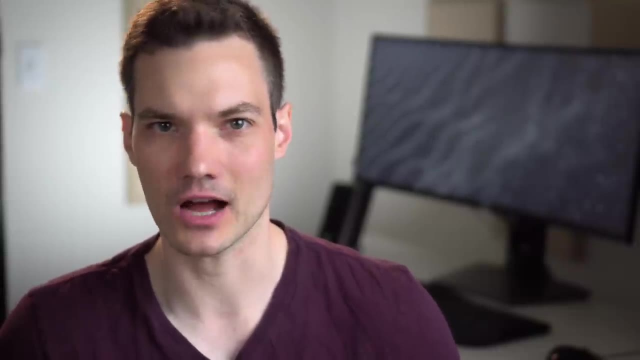 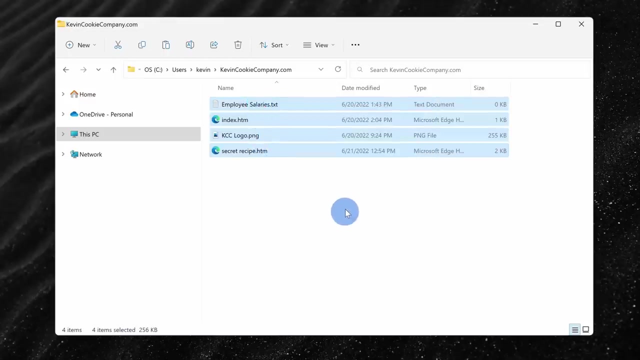 Once you've installed Git, you can use any terminal now to interact with Git. For this video, I'm going to use Git Bash, simply because it came with the Git installation on Windows. Here I am in File Explorer and I have these four different files that make up the kevincookiecompanycom. 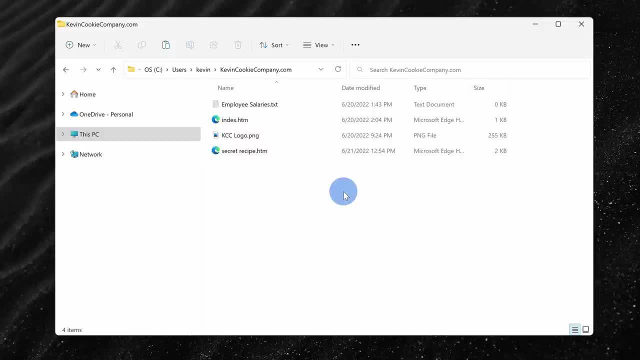 website. If you would like to follow along, you can download all of these files in the description of this video. Thanks for watching and I'll see you in the next video. Bye, I want to use Git for source control. So how do we do that? Well, let's open up Git Bash. 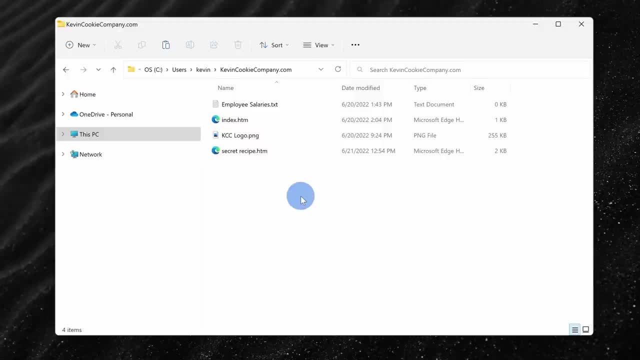 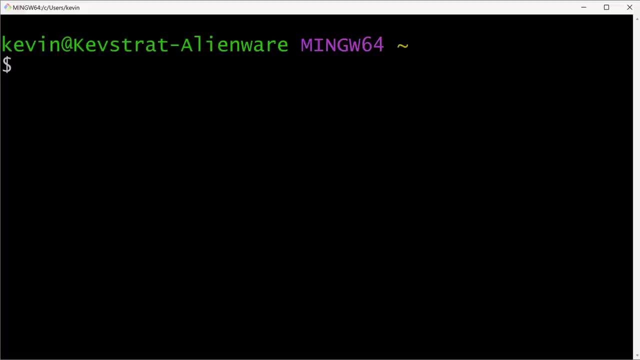 This is the terminal that we just installed. Now again, you could also use any other terminal that you would like. Here I am in Git Bash, and before we can get started, we have to configure a few things. First, we need to specify your name and also your email address, The reason this is so. 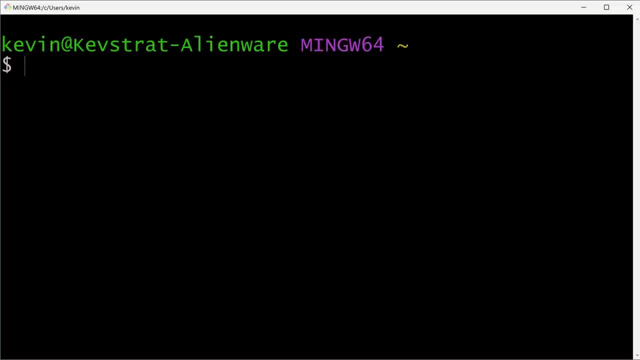 important is: anytime we commit something or write something to the history book, we need to know well who's doing it. First, let's specify the name Here. type in git config dash, dash, global user dot name. then insert quotes and here you can type in your name. I'll type in Kevin. 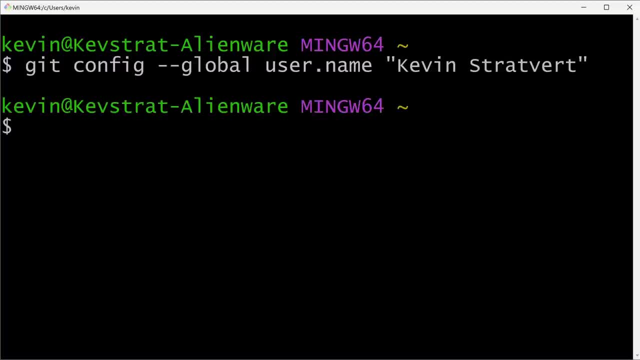 Stratford, and then close my quotes and then I'll press enter. Next we also need to specify your email address. Here let's type in git config dash dash global user dot email and then type in your email address. I'll type in: Kevin Stratford, YouTube. 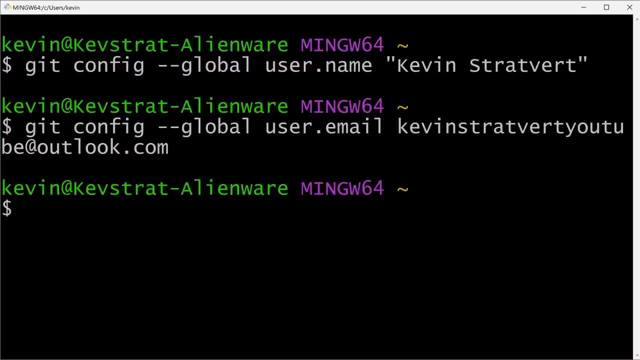 at outlookcom and then hit enter. Next, we also need to set the default branch name, and that might not make that much sense right now. Later on we'll talk more about what branches are and why you might want to use them, But for now let's once again type in: git config- dash, dash. 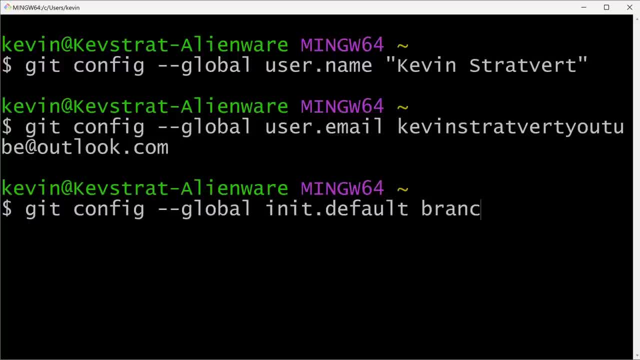 global init or initialize dot default branch and we're going to call the default branch main. Once you type all of that in, let's once again press enter. So far we've been using a command called git config and, as we're going through this, if there's ever a command and you're not, 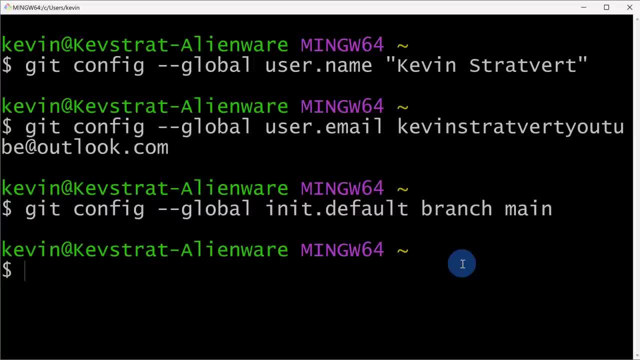 quite sure what it does or what different options you have for that command. you can very easily ask it for help Here. for example, I could type in git config and then I could type in a dash with an h. When I press enter, this will show me help. information about git config. Now zoom out a. little bit more, and here you can see all the different ways that you can get help with profit. Now, listen, let's zoom out a little bit more, and here you can see all the different ways that you could get help with profit and get help with get. 분들이 comes right after this and you can type in: git friend. 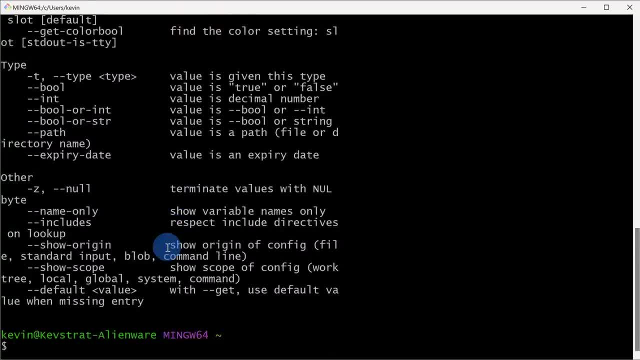 this will give us an ID, which is git. that tells you a –how you register. What's all the information can configure things Down below as well. if you want more detailed help information, you could also type in git help and then the command config. Here I'll press enter. 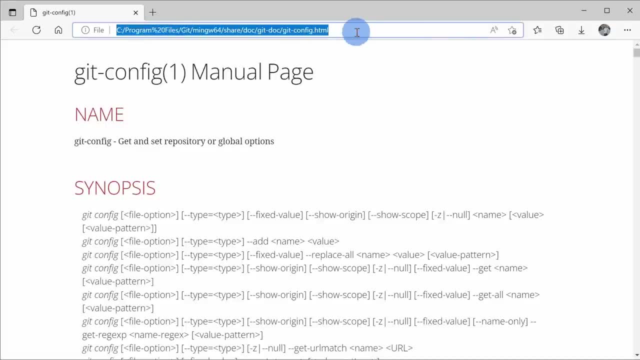 This opens up a manual that's hosted on your computer, so even if you're on the go or you don't have internet access, you'll still be able to access this file, And here it tells you more information about what that command does, and here you can see a full description of what it does. 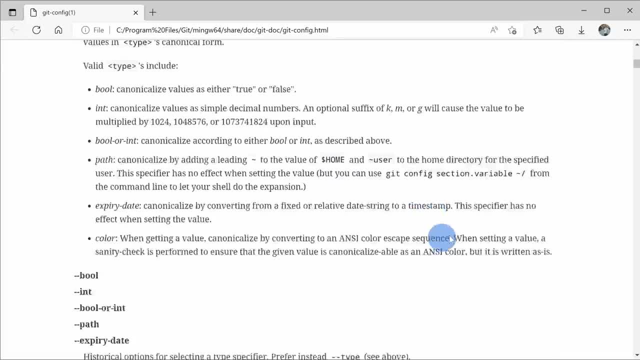 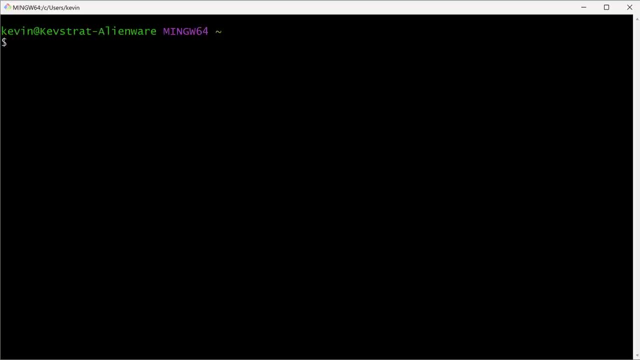 and you can see all the different options that you have when you run this command. Back now in the terminal to clear it out, the easiest way to do that is you could simply type in clear, press enter, and that gives you a fresh view once again Here, once again. 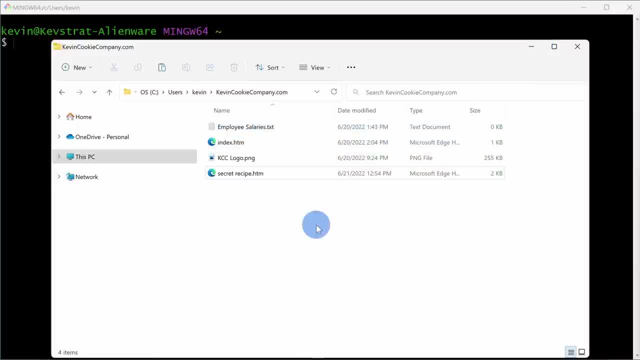 I have the following directory with all of the files that make up the Kevin Cookie Company website, and I want to use git to track these files. So let's take a moment to look at this address here and just remember where all of these files are stored. It's likely in a different. 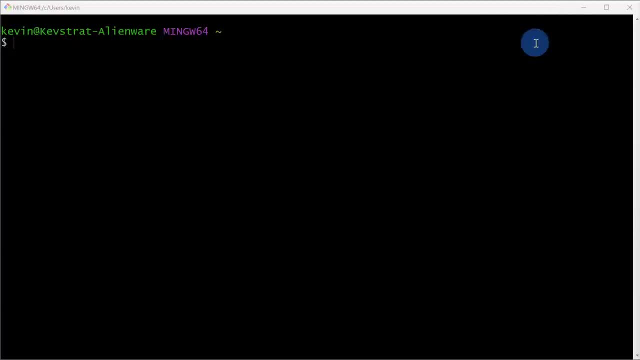 location on your computer, so just make note of that. Back here within git bash. we need to change the name of this file. If you want to change the name of this file, you need to change the name of this file. If you want to change the name of this file, you need to change the name of this. 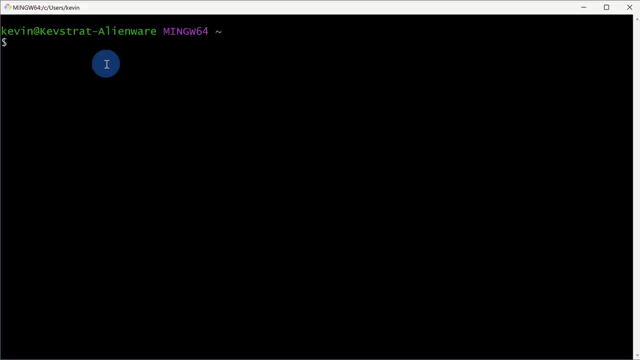 file. If you want to change the name of this file, you need to change the directory to look at where we have those files. To change the directory, let's type in cd that stands for change directory and then let's type in the location I have it in: c, colon forward slash. 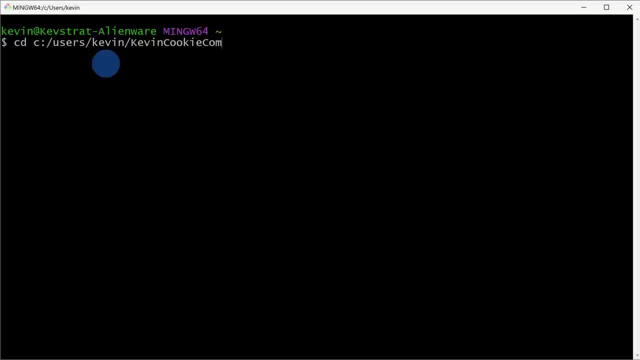 users forward: slash, Kevin and then KevinCookieCompanycom. Now I could press on enter and here we see that it's now looking at this location on my computer. To now turn this into a git repository, I simply type in git, initialize or I-N-I-T, and then I could simply press. 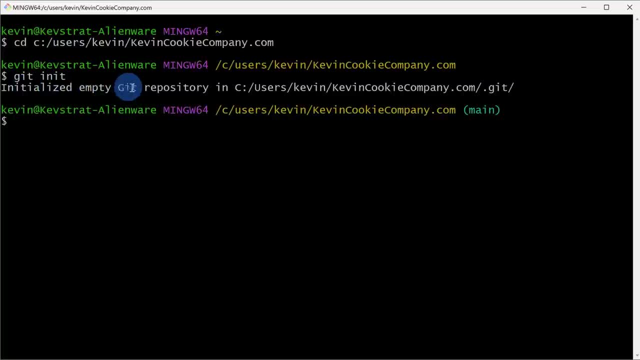 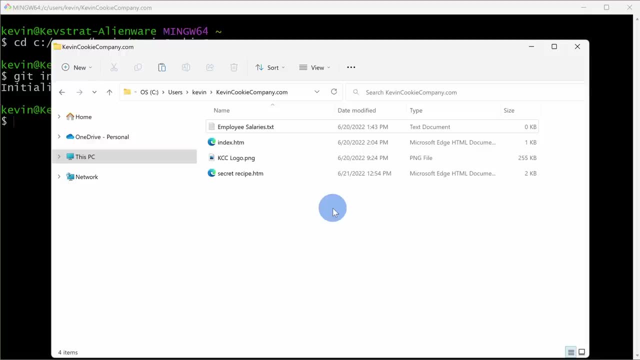 enter and here we see that it's now initialized this repository. Look at that. we've now created our very first repository. Back within file explorer it doesn't look like anything changed, but here, if I click on view and I'll go down to the option that says show: 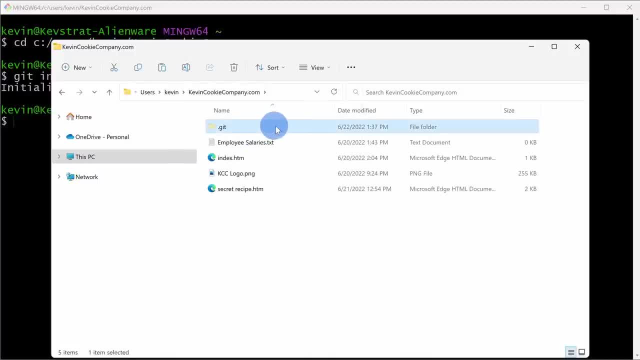 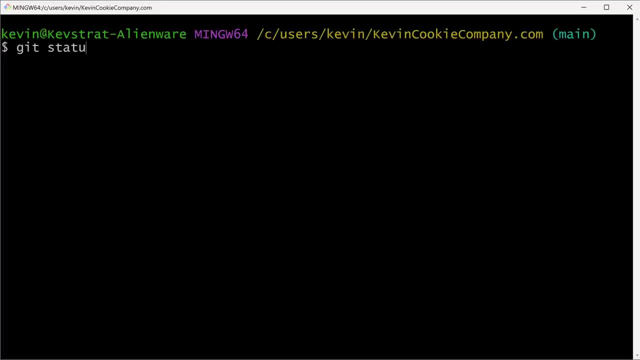 and here I can show hidden items. and here there's now a new folder called dot git. I can now click on that and this contains all the necessary repository files. Back within git git bash, we're now going to enter a command that you'll likely use often: Type in git status. 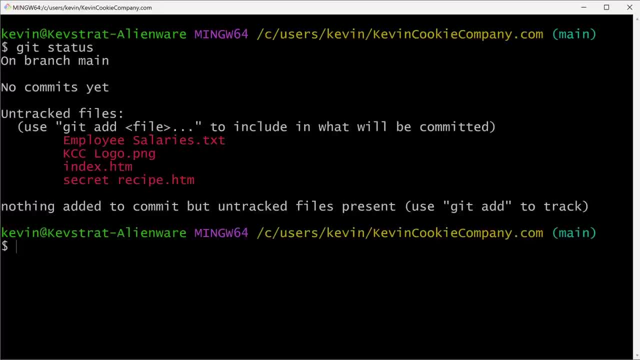 and this will tell us the status of our repository. When I press enter here, I can see that I'm currently on the main branch. Remember, at the very beginning we set main as our default branch. Here I can see that there are currently no commits yet. and don't worry, we'll get into what. 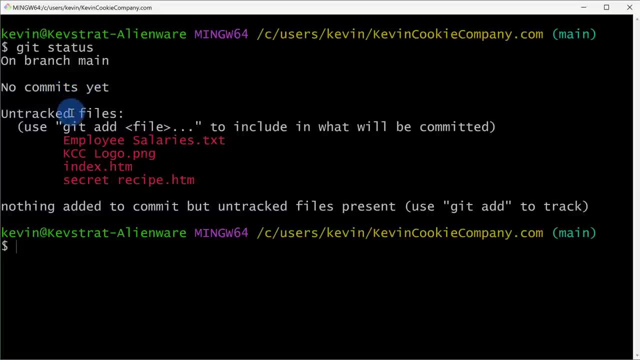 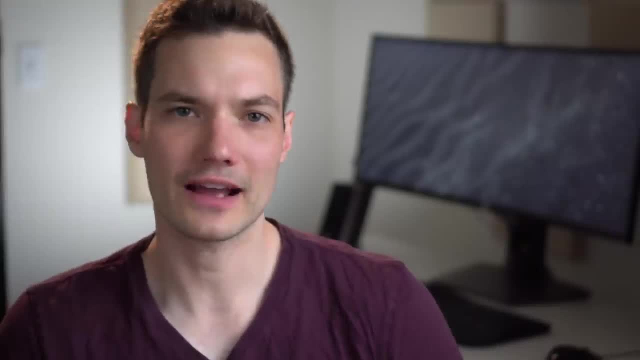 that is in a little bit, And down below I see that there are currently four untracked files. These are all of the files that I've been using to create this repository, So I'm going to go over all of the files that we saw in file explorer. Currently, all of my files are untracked. 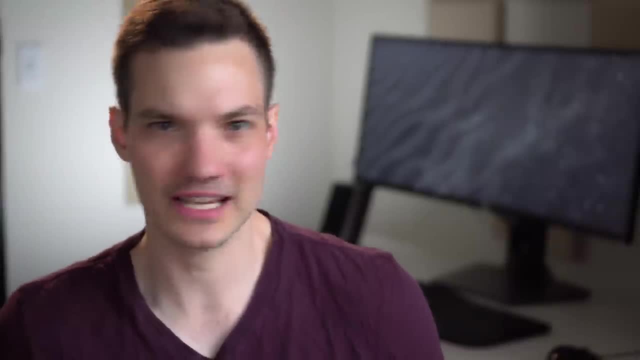 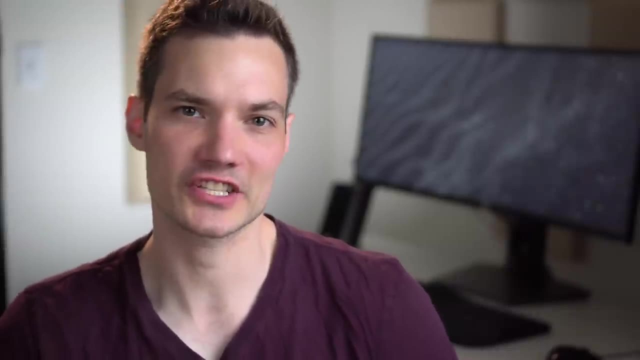 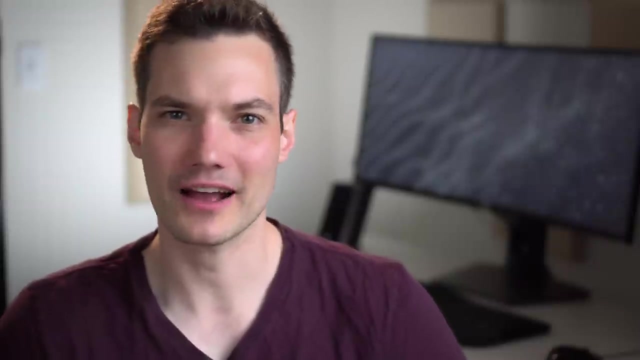 That means if I make any changes to any of these files, git won't care because they are untracked. Now if I track a file, git will know what changes I make to that file. So let's say I want to revert back to a previous version. I can do that. So how do we track a file? 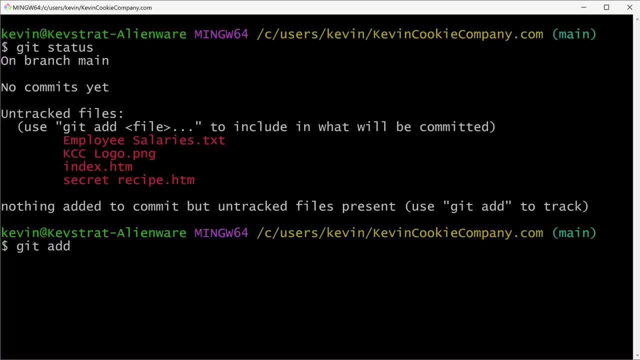 To track a file I could simply type in git add and then I could specify the file name. So let's say that first I want to track the indexhtm file Here I'll simply type in indexhtm and then hit enter. So this file is now being tracked. To confirm that it's being tracked: 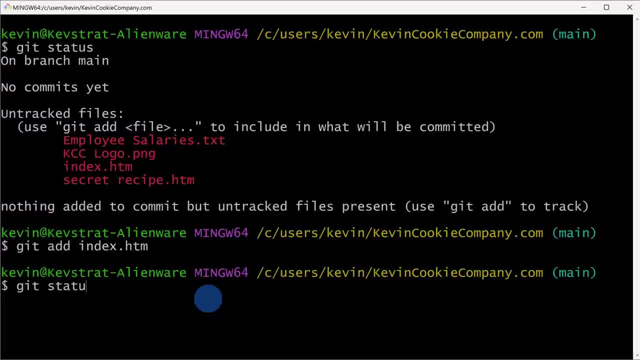 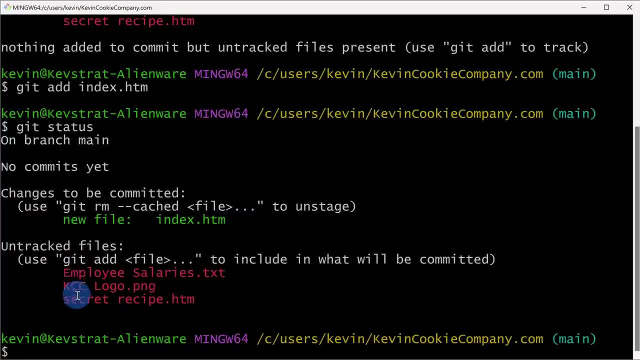 once again, we could use the command that we used earlier. I could type in git status, hit enter. and here I see that one file is currently being tracked and we continue to have three untracked files. Now let's say that, for whatever reason, I no longer want to track a file. 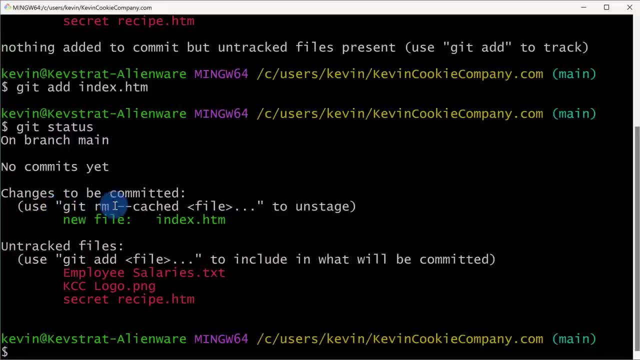 Right up here I see the tracked file, and right up above that I see a command that I can use to unstage or basically untrack this file. I could type in git rm for remove dash dash cached and then the file name. So let's try this out. I'll type in git rm- dash dash cached and here let's. 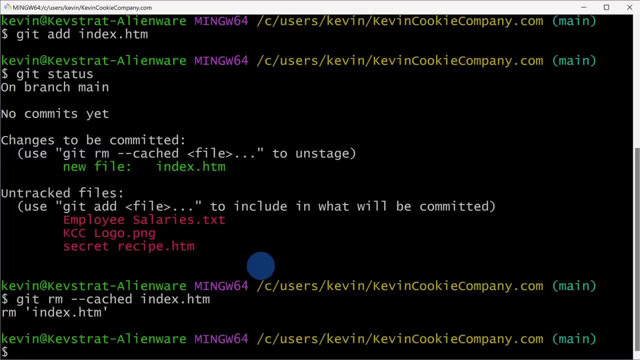 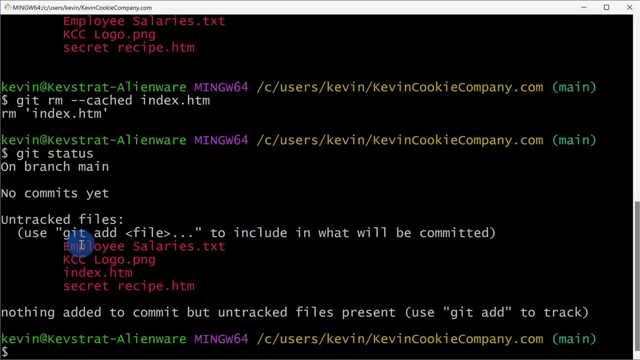 type in indexhtm, then I'll hit enter. Now once again, let's type in git status, hit enter and once again we're back to the original state, where all four of my files are currently untracked. I look at all the different files that git knows about Here. one of the files is called. 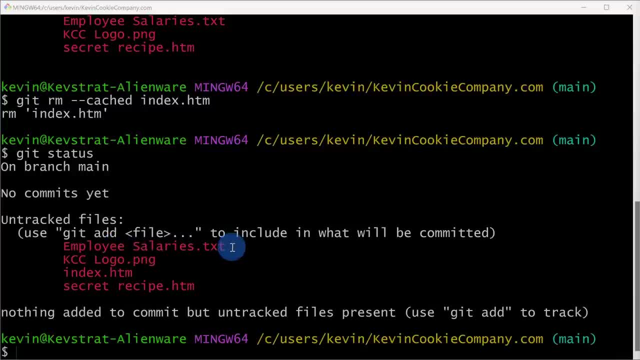 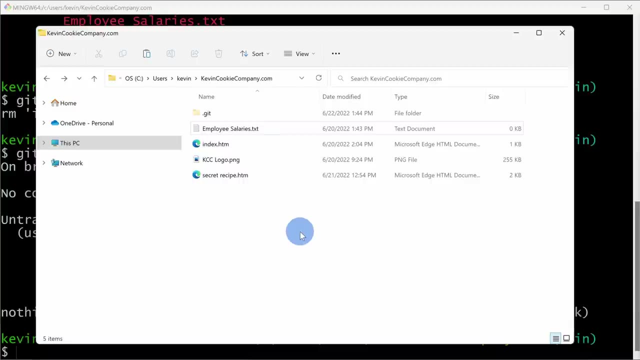 employeesalariestxt, and I definitely don't want to risk having anyone see this file. In fact, I would prefer to have git just completely ignore this file. Let's open up file explorer to see how we can ignore it. In file explorer, we're going to create a new file called 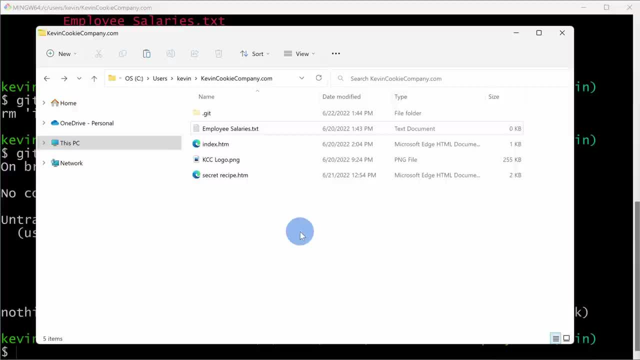 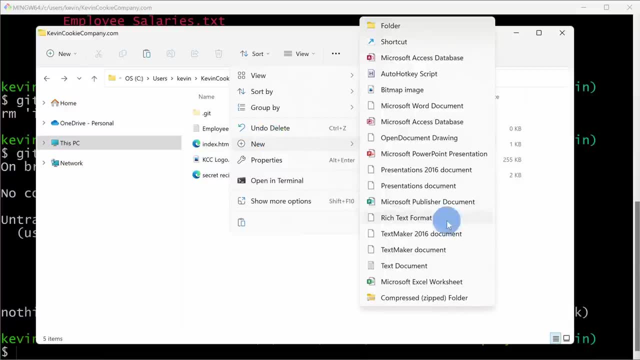 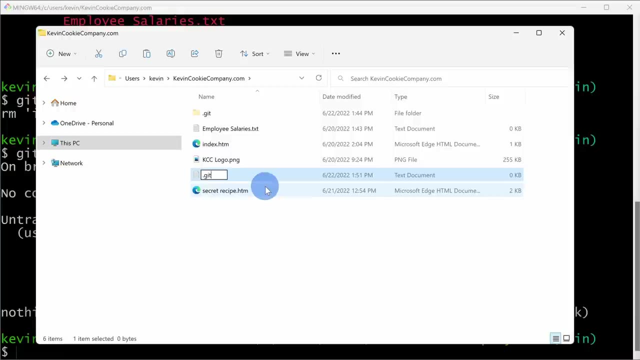 gitignore. This allows us to ignore certain files, folders or even just entire extensions. Here I'll right click and let's go to new and I'll create a new text document Right here. let's select the name and the extension and let's retitle this gitignore and then hit enter. 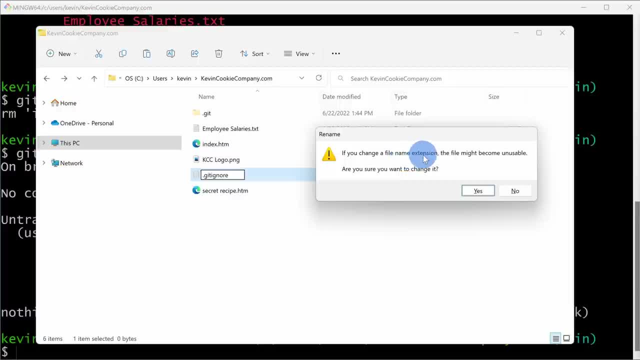 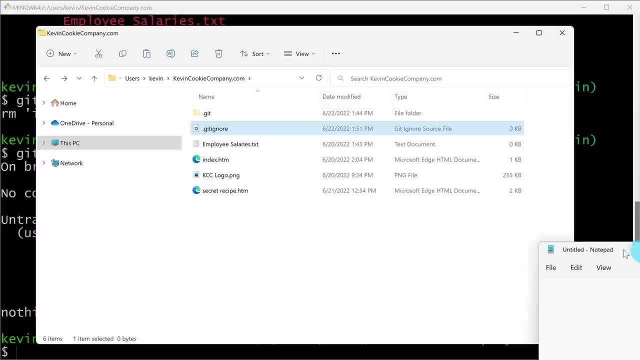 Here it tells me that it might become unstable if I also change the file name extension. Let's click on yes, And here I have a new file called gitignore. I'll take notepad here and let's open this file in notepad, or you could use whatever text editor you want. 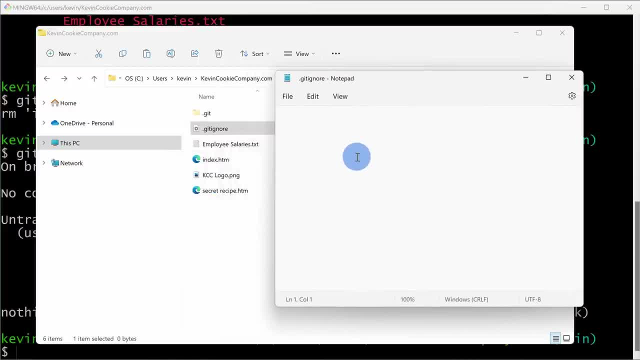 And currently there's nothing in this file. so I need to tell git what files or folders that I want to ignore. Here. I'll add a comment by entering in the hash symbol and I'll type in: ignore all txt files. Remember, the employeesalaries is a txt file. 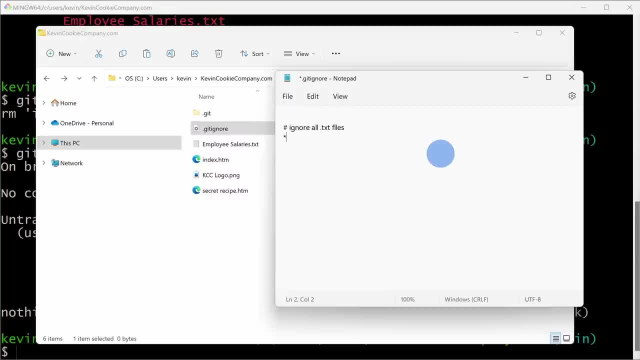 Underneath that here I can type in an asterisk, so basically any file name, txt I want to ignore. Now I could go to file and save To see a comprehensive list of all of the different ways that you can ignore files, folders or even just entire extensions. 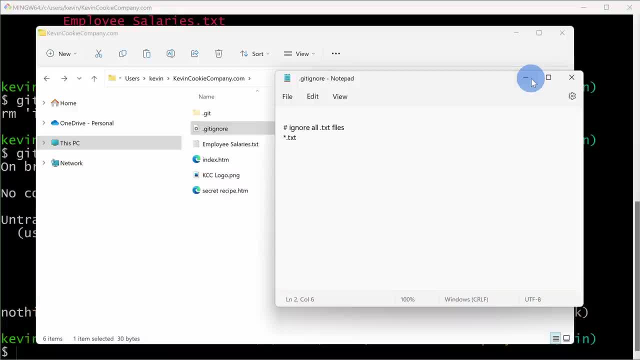 you could go to the website down below. This is ideal for things like log files or auto-generated files that you don't want to include as part of your project Or, in this case, maybe you just don't want to show employee salaries Back within git bash. let's see if git is in fact ignoring that file Once again, just like we've. 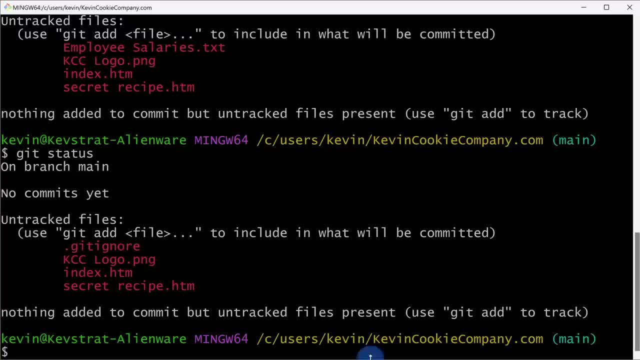 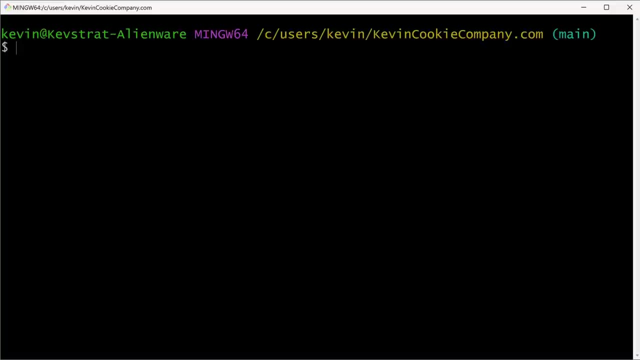 been doing all along. we can type in git status and then hit enter, And here I no longer see employee salaries. I really dodged a bullet there To give us a little bit more space. let's clear out this view. Now that we're ignoring one of the files, I want git to track all of the other files Earlier we. 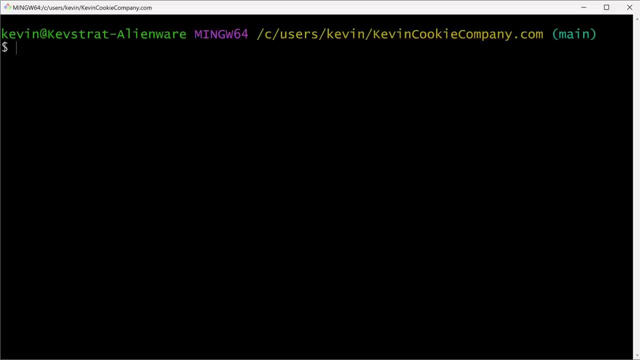 tracked that one file, indexhtm, but then I also untracked it. So how do I just track all of the files Here? I could type in git, add dash, dash all, and that'll track all the files. Alternatively, I could also type in dash capital A, or I could even simply type in dot for the entire directory Those. 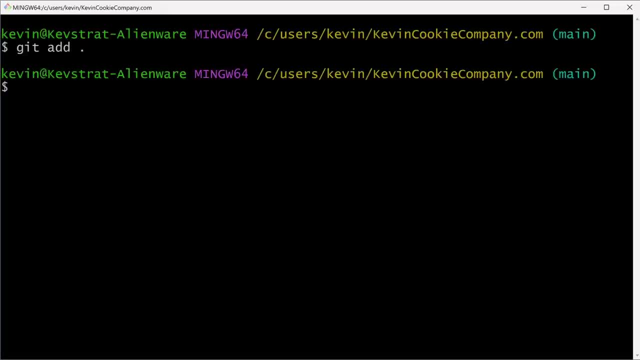 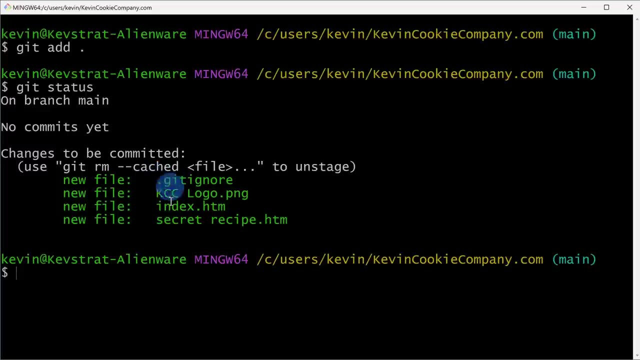 are all different ways that I can track all of the files Here. I'll press enter and let's check what happened Once again. let's type in git status, hit enter and here I can see that all of these files are currently being tracked, except for that file that I ignored, And currently all 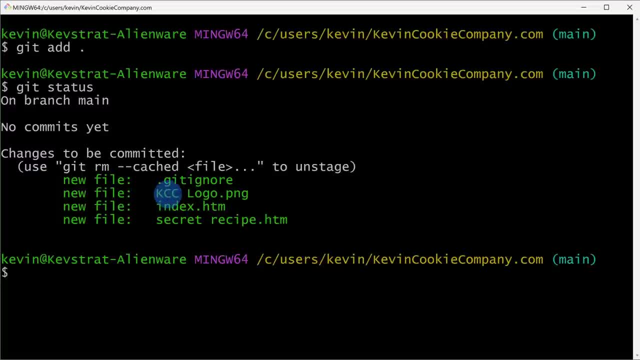 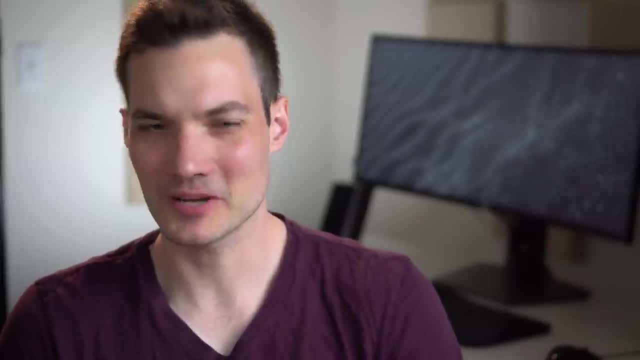 these files are in an environment called staging. Now that I've added all of these different files, I want to commit them. So what does it mean to commit? To commit: you're taking a snapshot of your repository at this point in time, basically what all of your files look like right now. 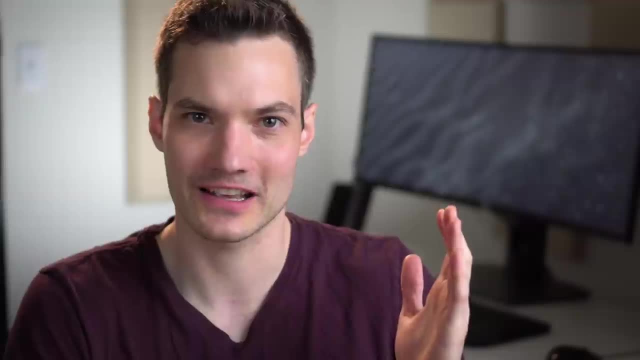 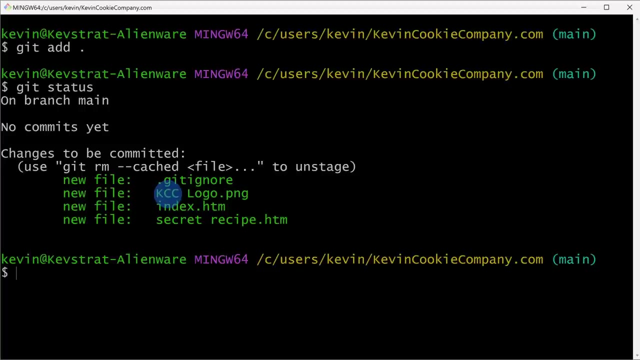 In a sense, it's like writing an entry into a history book, and if you ever want to go back to this point in the future, you could do that. To commit them, we could use the commit command. I'll type in git, commit, dash m and then open quotes, and here I can type in a message. 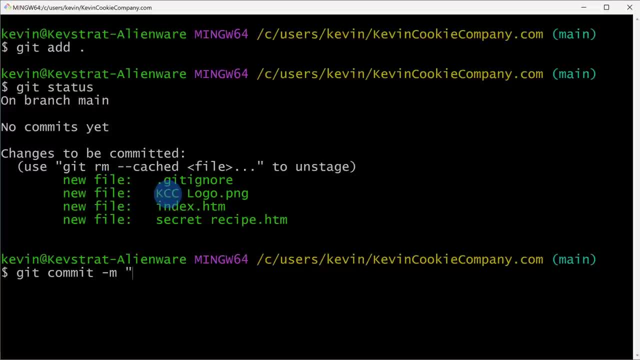 to go along with this commit. Now, remember, when we commit something, that's like writing the current state of all of these different files to the history books, and this message will go along with that entry. Here I'll say: this is my first commit. 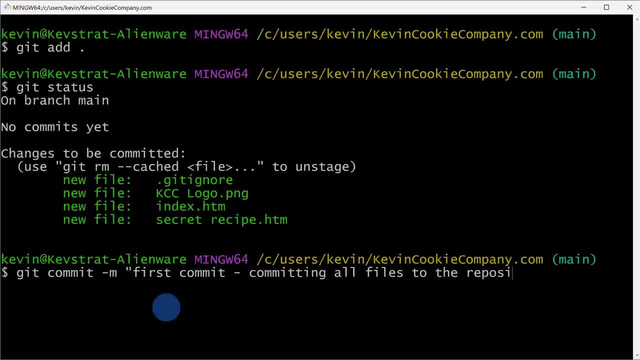 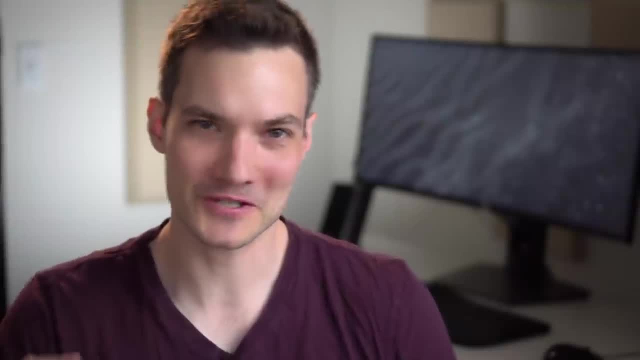 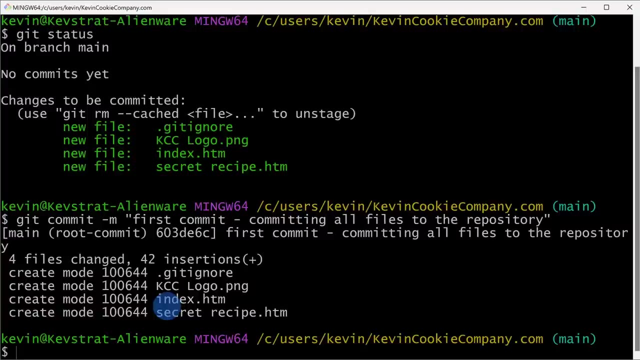 and, let's say, committing all files to the repository. Then I'll close my quotes and here I could press enter: Congratulations, you just finished your first commit and there's now a page in the history books. That wasn't so bad, was it? And just like that I've now committed all four of these. 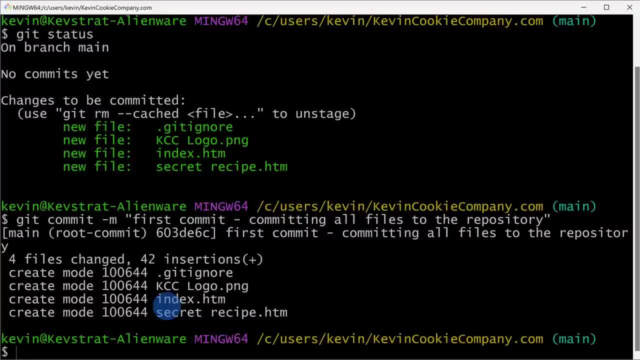 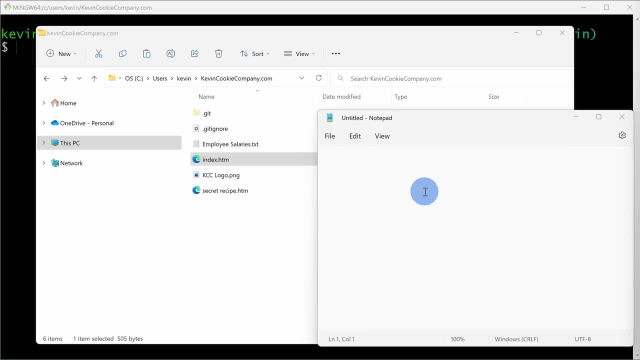 files and they are now officially part of the git record. Here I could type in git status once again and I see that there are no longer any files to commit. Let's say, I now want to change one of my files. I want to modify the indexhtm file. 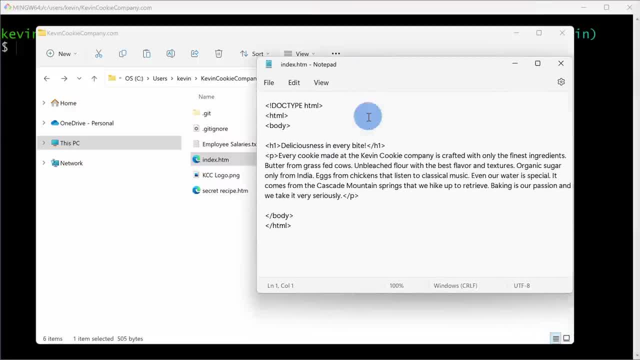 Here. I'll click on this file and I'll drag it into Notepad. and here we see the contents of the file. Now, if you remember, we say eggs from chickens that listen to classical music, but I've recently found out that that's actually not true. 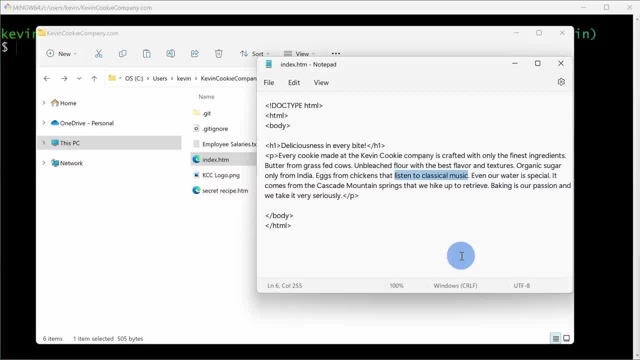 So let me remove this reference and maybe we just say that our, let's say, free range, and next I could go up to file and I can now save this file Back within git. I can now type in git status, hit enter and git recognizes that one of 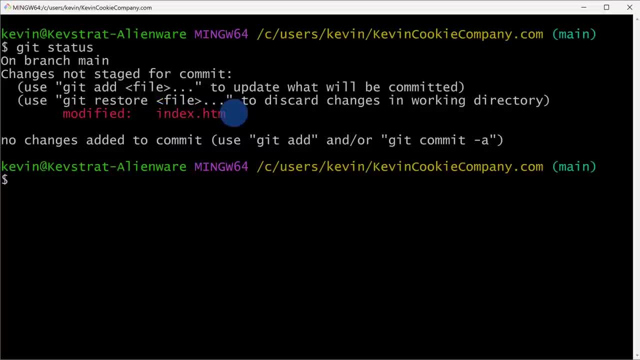 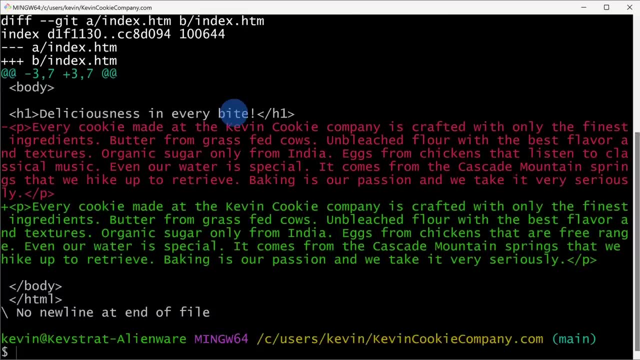 these files has been modified. To see what's been modified, git has a command for this. We could simply type in git diff and this will show us what the differences are. I'll hit enter And right here, if I scroll up just a little bit here, we can see what the file name is. 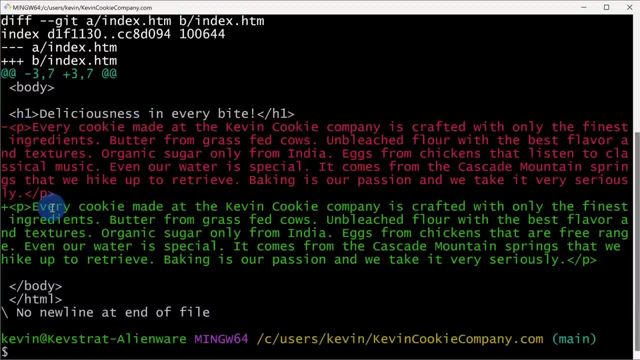 and here I can see the original text in red and here I can see the changed text in green. So once again the red text shows that listen to classical music and down here in the green text we see that our free range. I'm satisfied with all of these changes and once again I want to add this change to the. 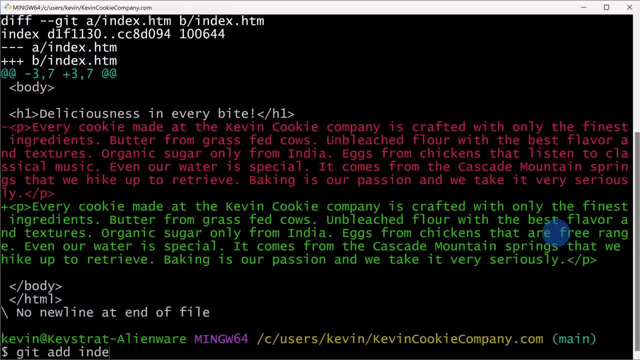 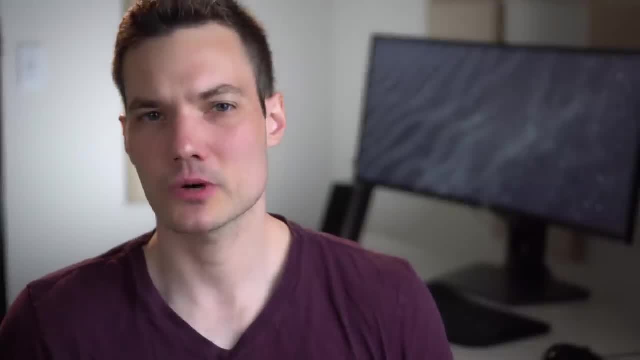 history books. Let's once again type in git: add indexhtm. The file is now correct. It looks like it'sExit. Here's what it looks like after adding in a change. So in git you've already defined the state and once again, it more than atrás. 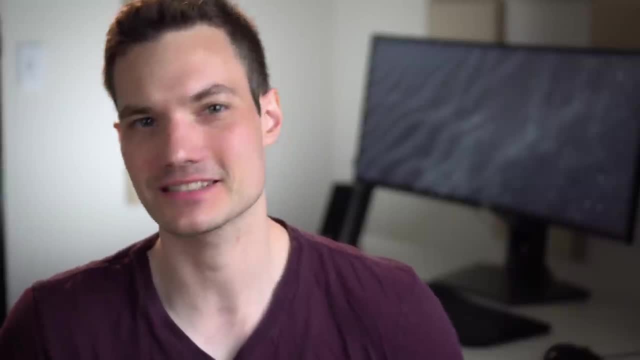 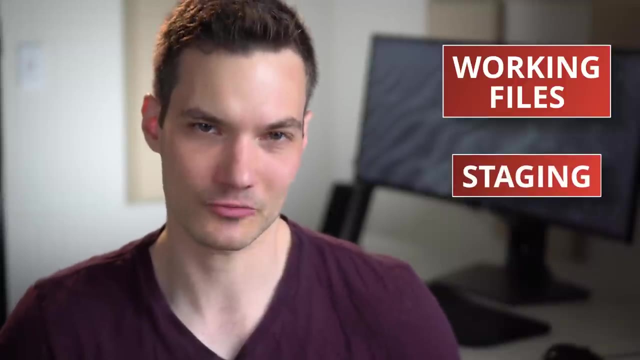 You just need to click confidentially and click on see what's actually happening with it. And now, if I would click to edit the six pieces, we can see now that it'sA10.. We're using several different versions and the answer we get is this: is this isn't an. 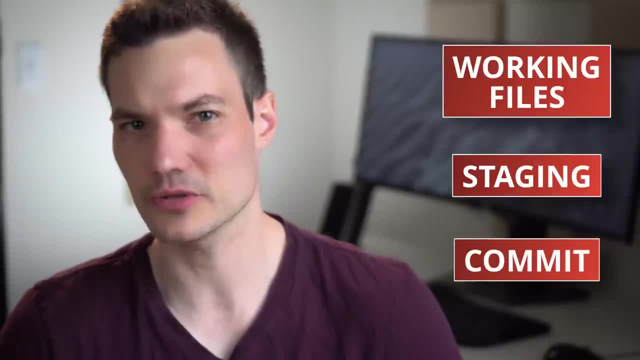 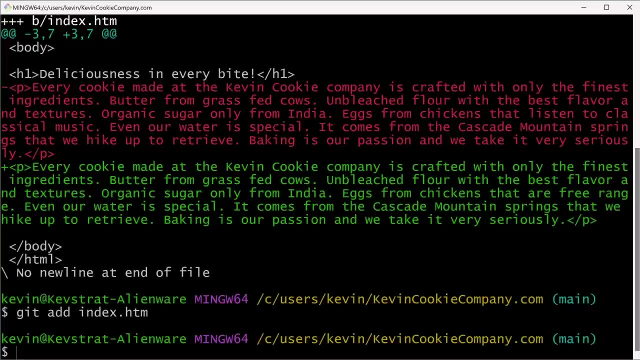 introduction to Git. this is a base term, So we're right here. There'll be subtitles from all over or where you commit things, and this has now been added as a log or an entry into the history books. Let's say, I want to remove this file from staging. Maybe I'm not ready to commit it. 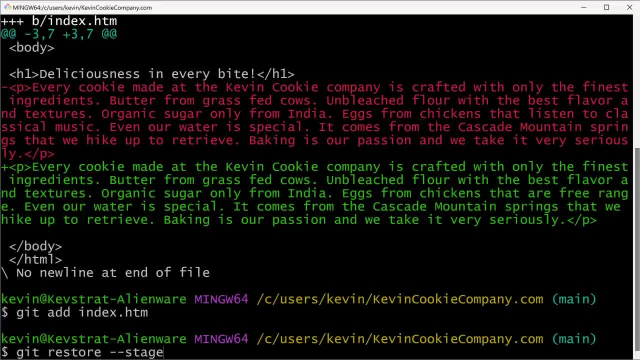 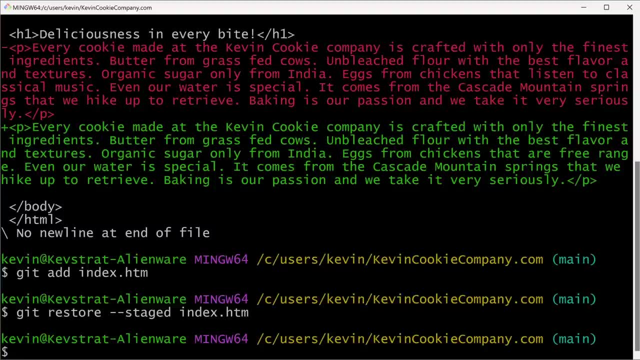 I could type in the command git restore dash, dash staged and then indexhtm. Now, once I press that, this moves that file back to my working files. So if I were to commit now, this file would not be included, because this file is currently in the working environment. 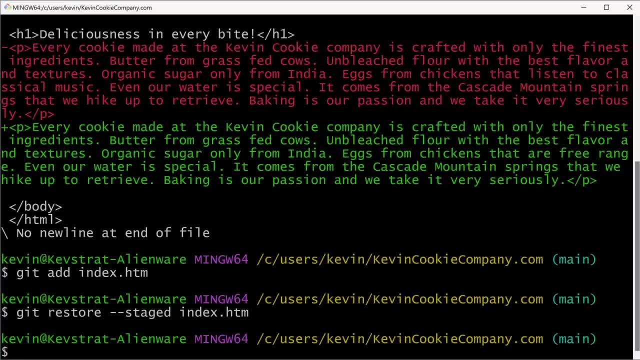 So let's say that maybe you're working on six files and let's say that three of them you're ready to commit. You can move those three to staging and then you could commit them and the files that are currently in the working files. those would not be included. The indexhtm file. 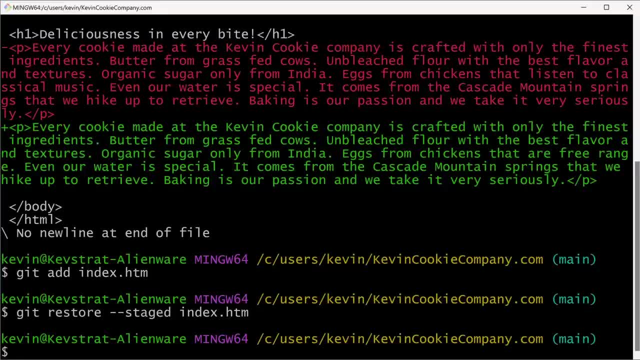 is once again in my working files, but I do actually want to commit it. So once again I could add it back to staging and then I could commit it from staging. But I could also just bypass or skip over staging altogether To do that. 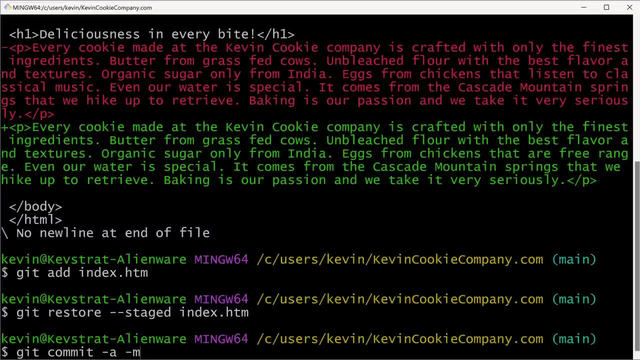 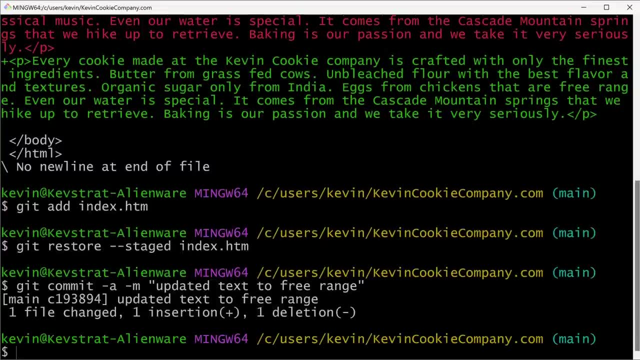 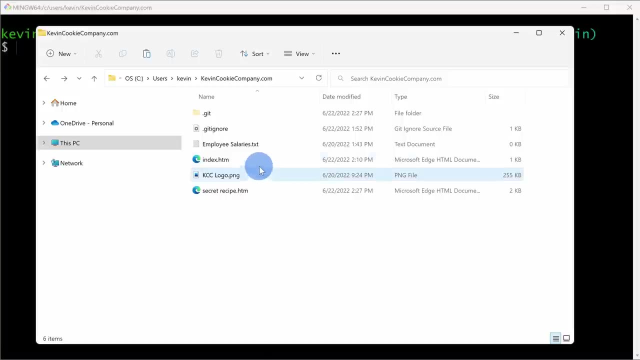 let's simply type in git: commit dash a, dash m, and here I could say updated text to free range. Then I can close my quotes And now, when I hit enter, this skips over the staging step and it's now committed this change. Here within my git repository I have one file called secret. 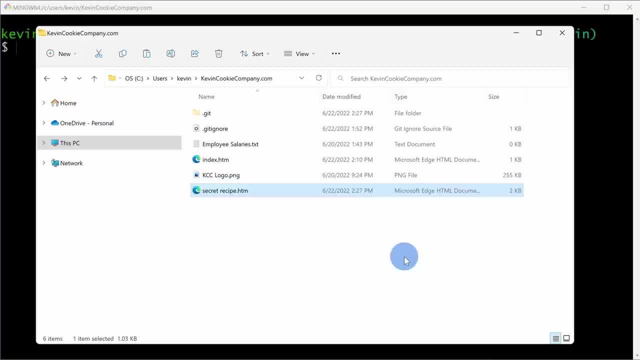 recipe and I definitely don't want that falling into the wrong hands. So I should probably do a little bit more work on that. So I'm going to do a little bit more work on that. So I'm going to probably just delete the file, and I could do that directly through git. I. 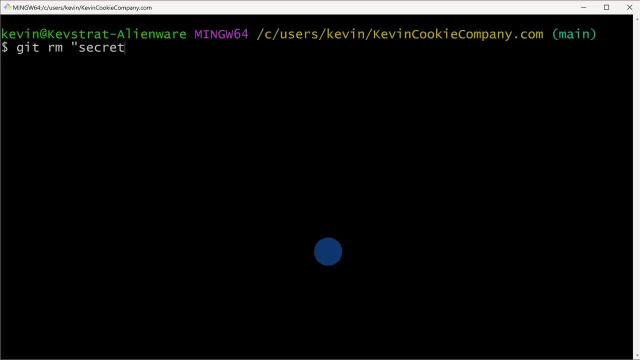 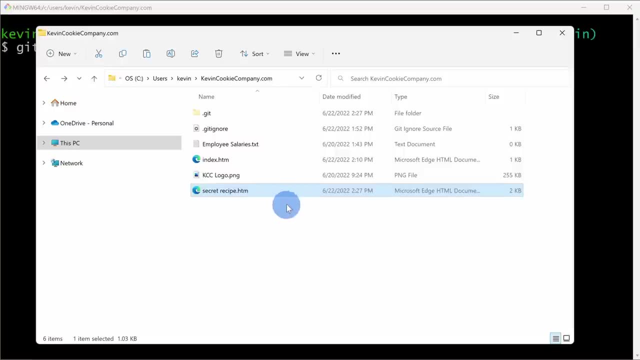 could type in git rm- rm for remove, and then I could type in the file name, secretrecipehtm, and then close my quotes. But an even easier way to do that: just directly in file explorer. I could also delete the file right here and now. that file is gone. 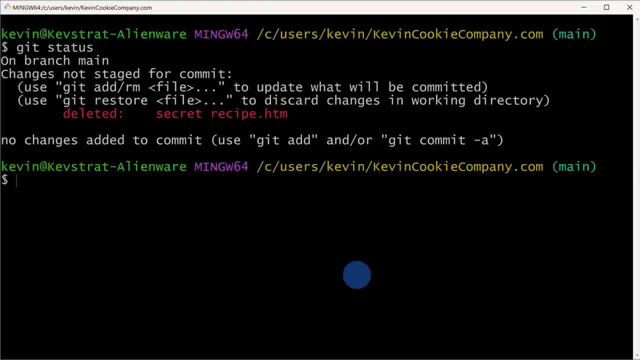 Back within the terminal. let's type in git status and then hit enter, and here git recognizes that this file has been deleted, and the reason why is: this is one of the files that git is tracking. On second thought, maybe I should keep this file. I personally haven't. 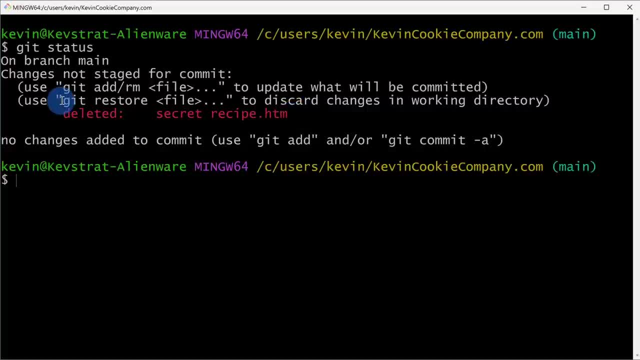 memorized the secret recipe yet, And right up here I see a helpful hint: If I want to restore this file, I could type in git restore and then the file name. So let's test that out. I'll type in git restore and here I'll insert quotes, and let's type in secretrecipehtm and then close. 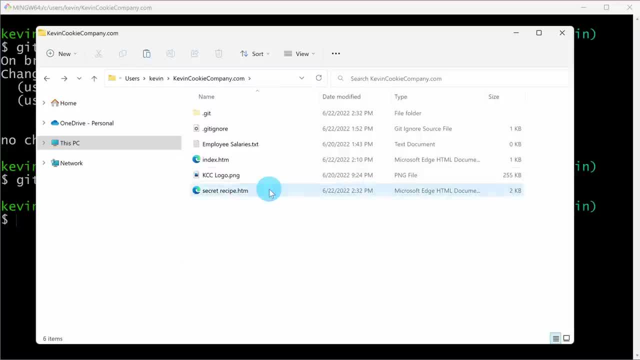 quotes and hit enter. If I go back to file explorer, look at that. The file is now back Now. once again, this is one of the advantages of working with git. If you've ever previously committed a file, you can always go back to a previous version or you can recover. 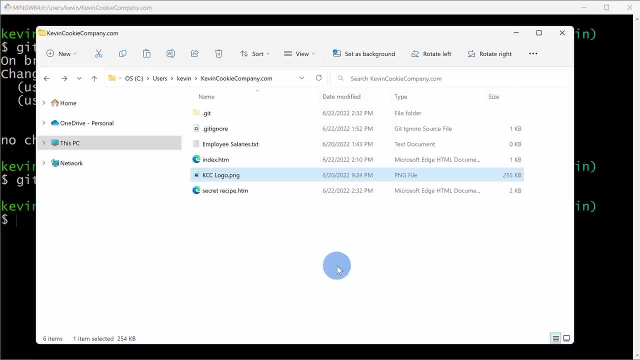 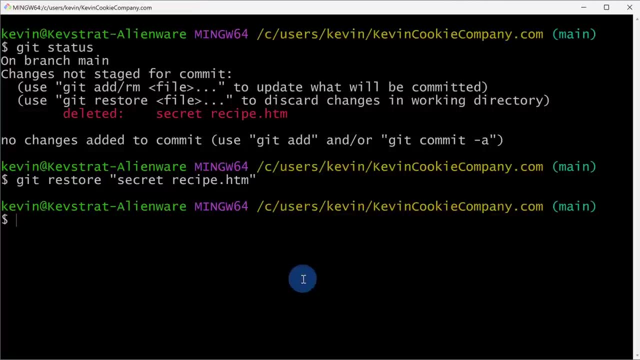 that previous version, if you need to. Similar to deleting a file. if you want to rename a file, you can either do that directly in file explorer or you can do that back in the terminal. Let's try renaming a file in the terminal. I'll type in: git mv and we're using mv and that stands for move. 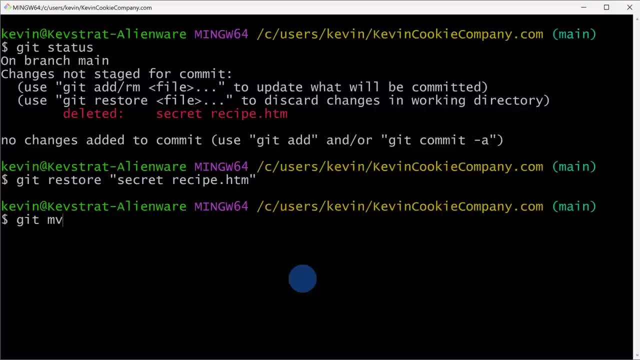 so we're basically moving from an old file name to a new file name. Here I'll type in the original file name and that's kcclogopng, and I want to move to the new name, primarylogopng. then I'll. 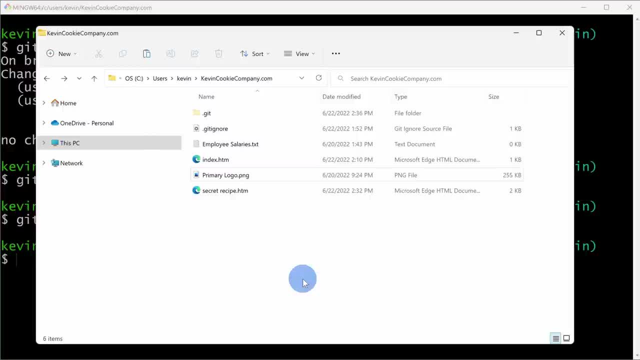 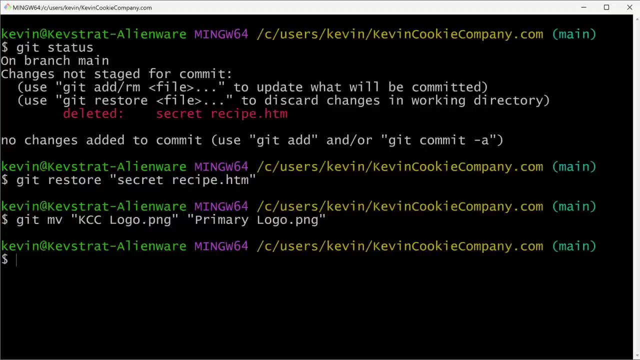 close my quotes and let's hit enter. If we go back to file explorer here I can see that the file name has been updated. I want to add this change to the history books. Basically, I want to type in git commit dash m, and then here I could type in the message. Let's say we changed. 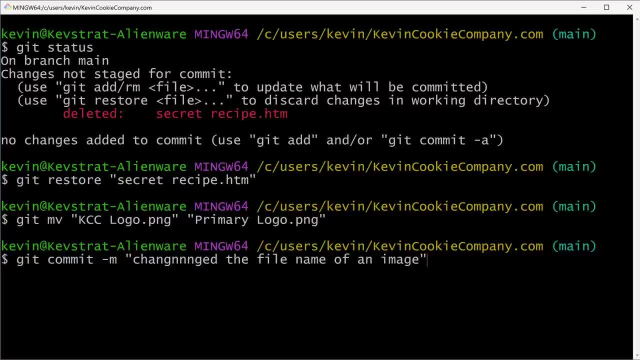 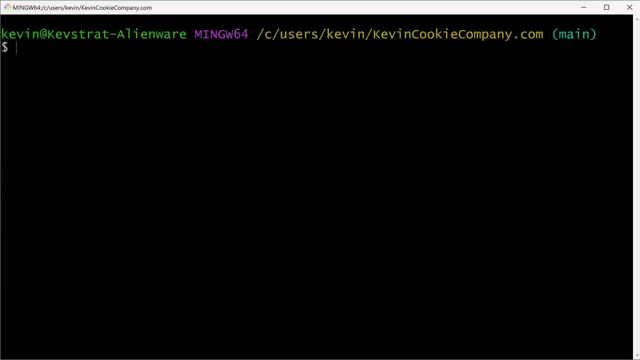 the file name of an image and then I'll close my quotes and here I could hit enter. and that has now been committed. So far we've made a number of different commits or basically entries to the history book or the log. What if we want to review all of the different commits that we've? 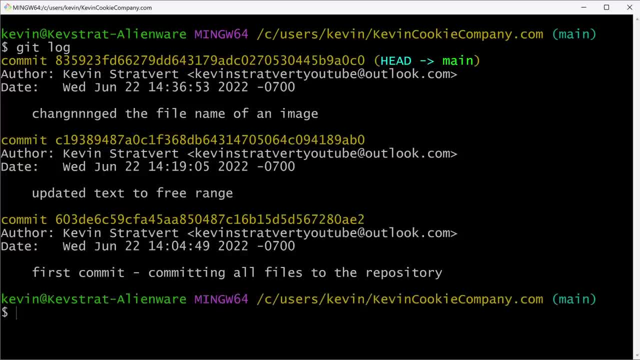 made. We could type in the command git log and then press enter, And here we see all the different commits. Every single commit has a unique identifier. Here we also see the author, And if you remember, at the very beginning we defined who the author is. 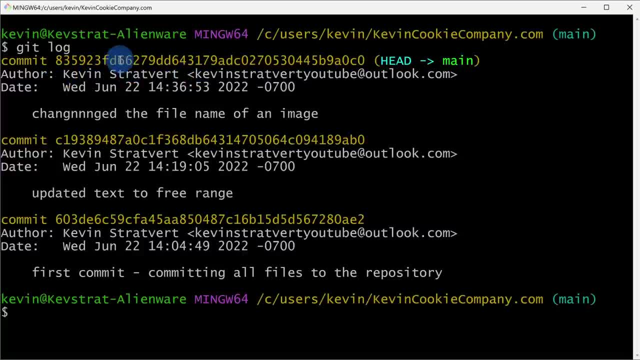 So I typed in Kevin Stratford and then we also typed in an email address. Then I could also see the associated date with this commit. So here at the top we go with the most recent all the way down to the oldest commits, And right here I could also see the text that I typed in as part. 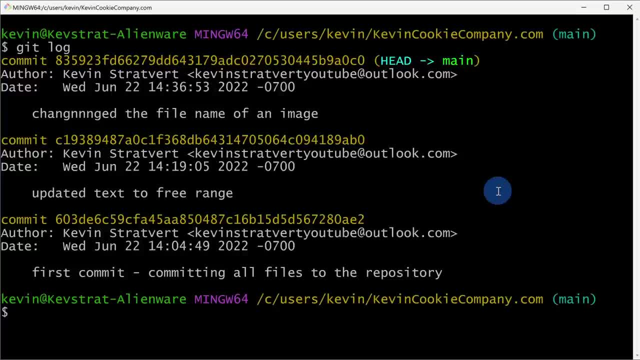 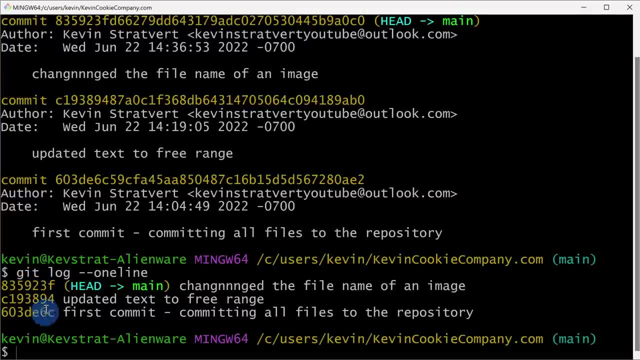 of that commit. If I want a more abbreviated version of this view, I could type in git log dash dash, one line, and then I could hit enter, And here we see an abbreviated version of all of the commit history. Now, looking at this commit history, I just noticed that I typed in this text incorrectly. 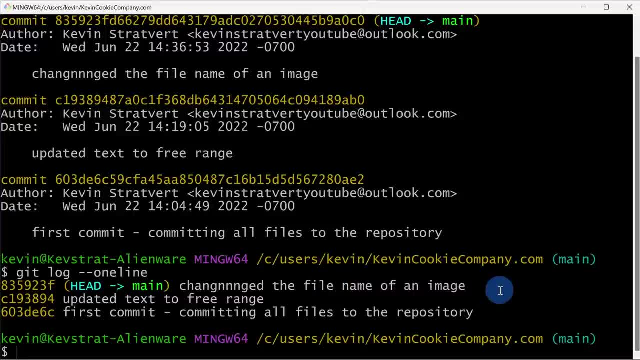 and I could go back and commit again and then type in the text properly. but I actually just want to amend that text. Luckily with Git we can do that. I'll type in git, commit dash M, and here I'll say: changed file name to primary logo dot PNG, and then close my quotes. 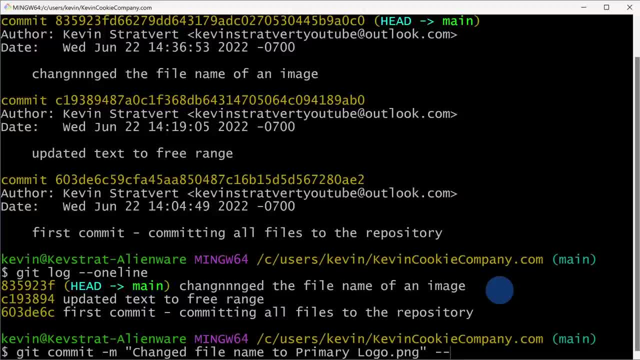 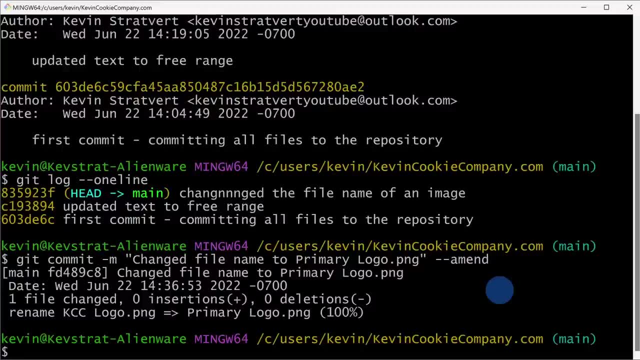 And at the very end of this commit command I could type in dash, dash, amend, and then press enter And that's now amended, that entry. Now here, I could press the arrow up icon on my keyboard and I could go through all the different previous commands that I've entered. I could go up to git. 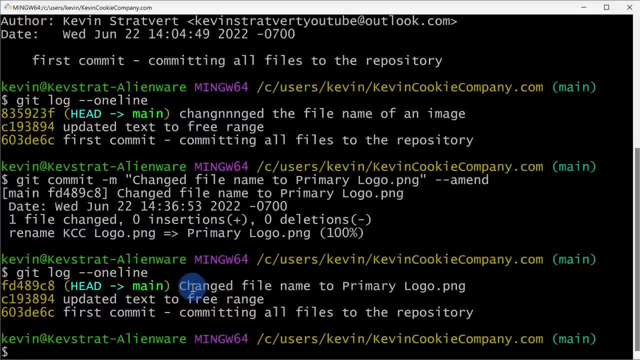 log dash. dash one line, hit enter and here you see that that text has now been corrected. So that's a really neat way that you can just go back and quickly amend a previous commit without having to submit yet another commit into the history books. I have all of these different 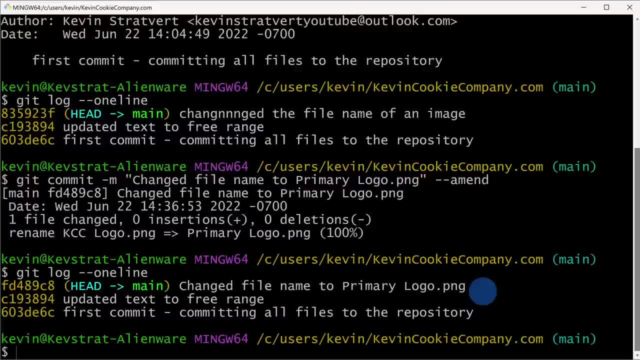 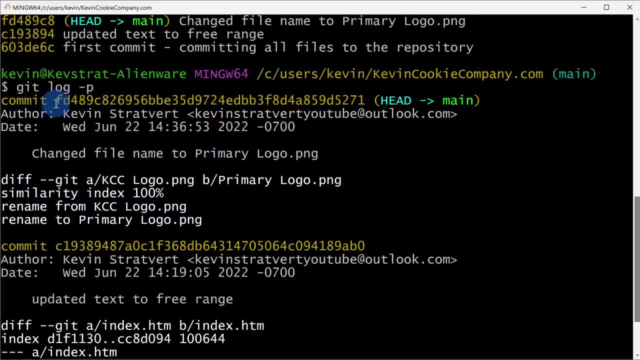 commits. but let's say I want to see what actually changed in these different commits. I mean, I have some text here, but what if I want to dig into these specifics Here? I could type in git log dash P and then hit enter And here I could look through and see all of the different changes Here. 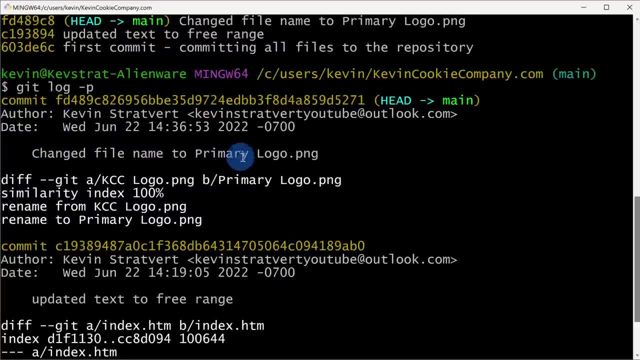 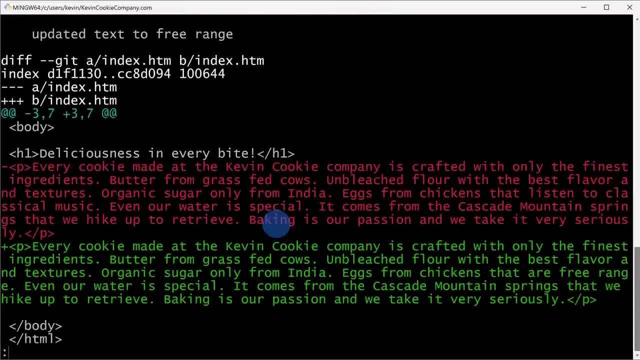 for example, I could see in the most recent commit. it's a file named to primary logo dot PNG, And here I could see that I updated text to free range and if I press my arrow key down here I could see what the original text was and I could see what. 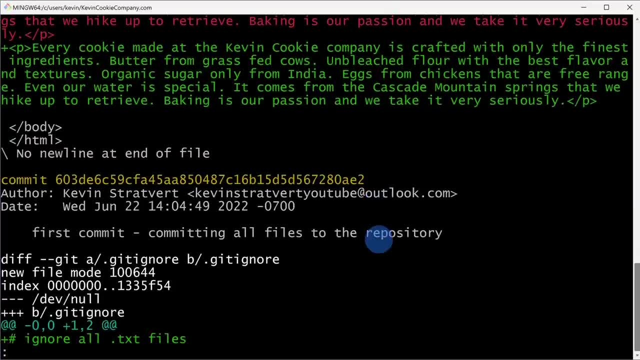 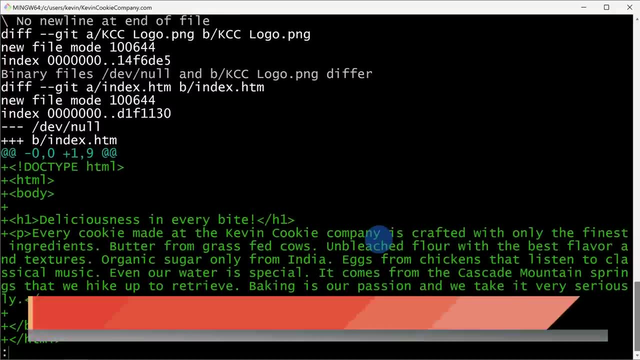 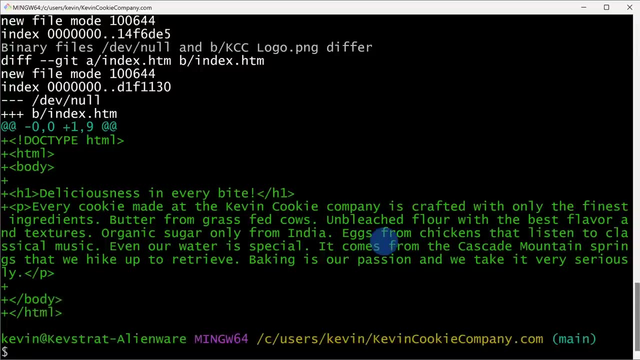 the new text was: And if I press my arrow key down some more here, I could see my very first commit where I added all of these different files to the git repository. To exit this view I can press Q on my keyboard- Q for quit- and that exits out of this view. Git log has all sorts of advanced. 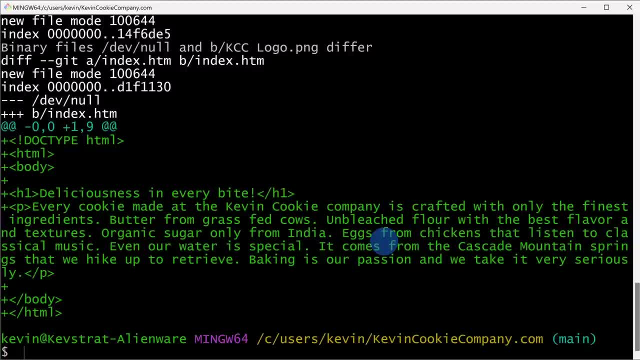 capabilities. You could search for specific text. You could look for changes that happen before a certain date or even after a certain date. Now, once again, as we looked at earlier, if you want to find out the full capabilities, you could type in git help log and then hit enter. 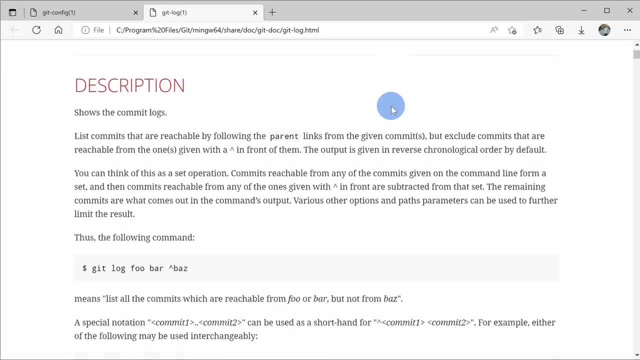 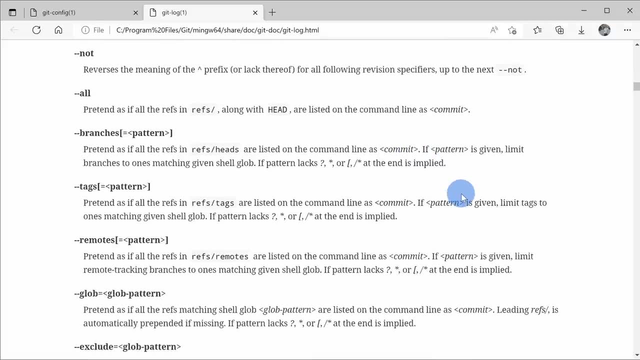 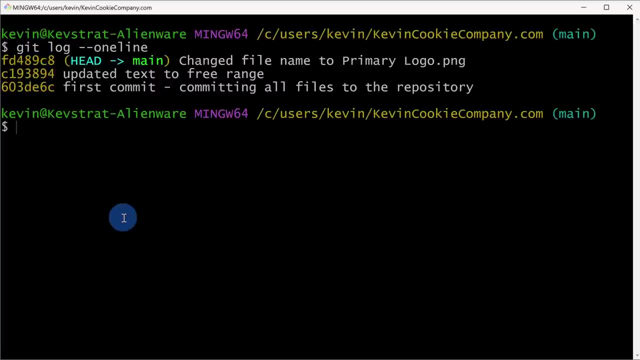 This once again opens up the manual for git log, and here you can see the description and here you could go through to see all the different capabilities of how you could find specific changes in your commits. One of the great things about having git history is you can always jump back to previous commits. To do that, you simply type. 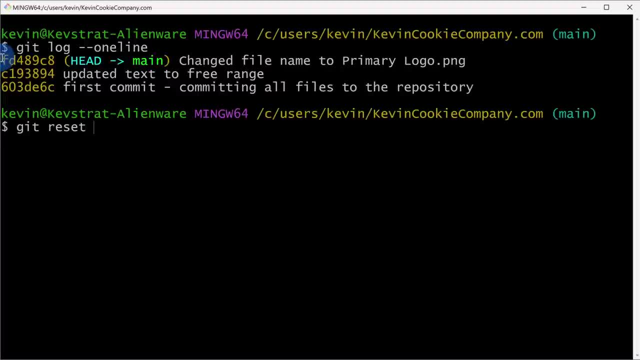 in git reset and then you can type in the hash tag. So here, for instance, if I wanted to jump to updated text, to free range, I could simply type in this value here, and that would bring me back Now. of course I don't want to do that, so I'm going to remove this. You also have the option to 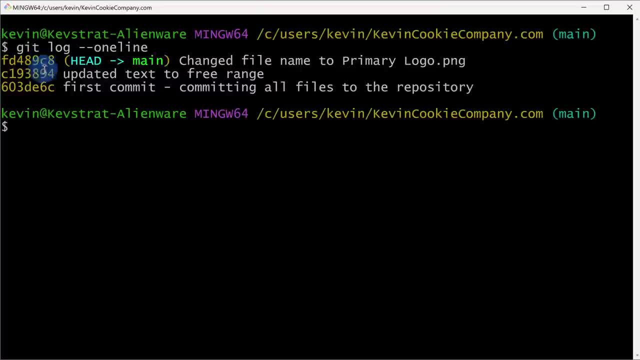 modify what appears in the history book and also the order in which all of these commits appear, and you can do that using something called rebasing. Here I could type in git rebase –i –root and then hit enter. This brings me into 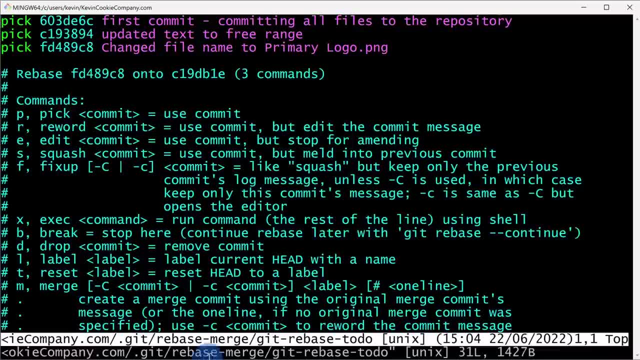 an editor. Here I see my three commits, and then I have all of these different options to modify the way things appear. Once again, I could change the order. I could even merge together or squash two of these commits. Now, this is beyond the scope of this video today, but I wanted to let you know. 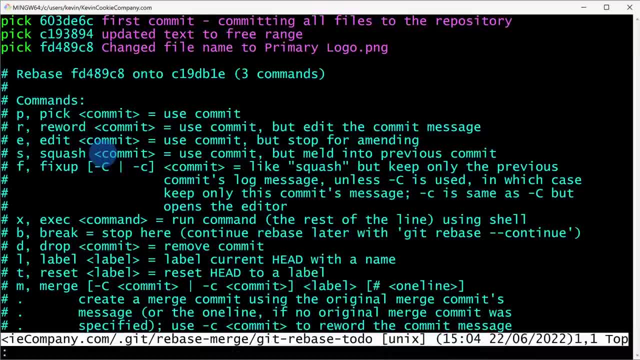 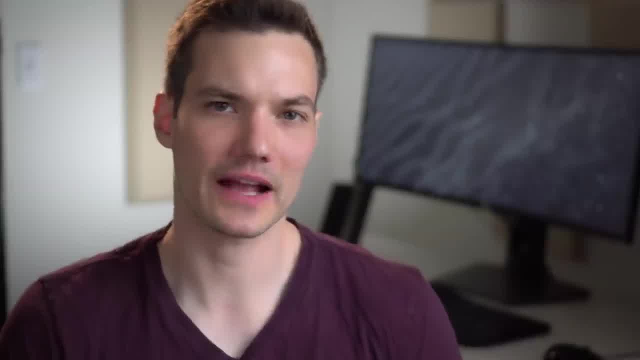 that this is possible. To exit this view, press the colon key, then X and hit enter, and that brings us back into the main terminal view. So far we've been making all of our changes just directly to the main branch, but you can also set up additional branches. 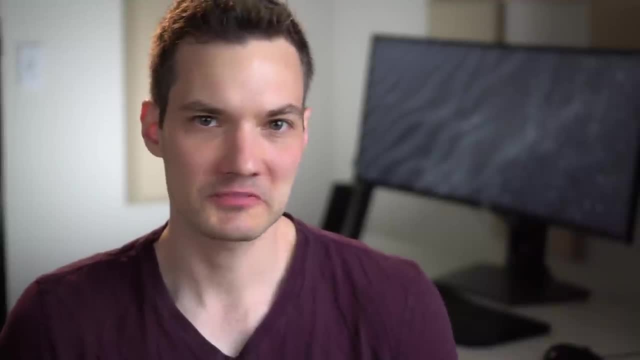 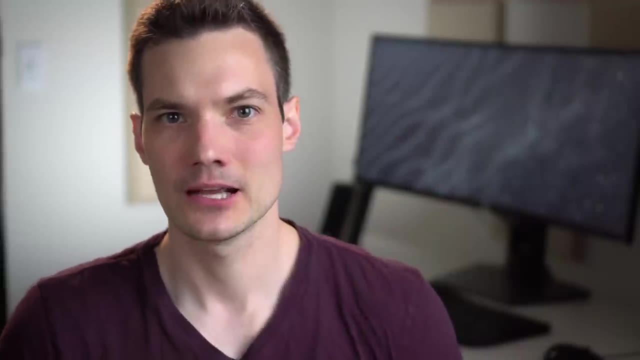 What is another branch? Another branch is basically a copy of your main branch and it has all the same entries in that history book, but this allows you to go off and work on, let's say, a feature, or maybe you're fixing a bug and you can make all your changes. 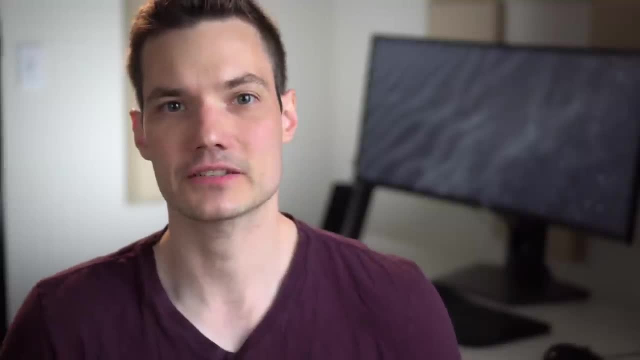 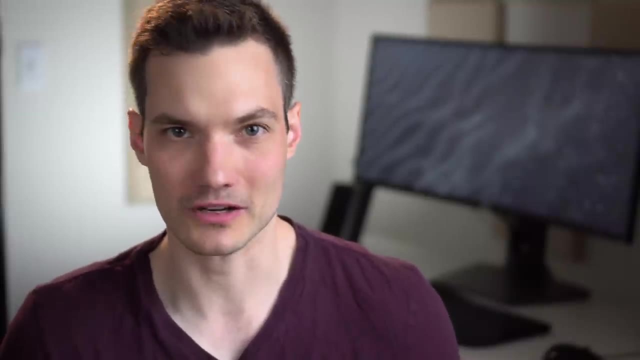 and it won't affect the main branch. Once you're satisfied with all of your changes, you can then merge it back into the main branch. This is also how software development typically works. You'll have developers and maybe one's working on a new feature. They'll create a new. 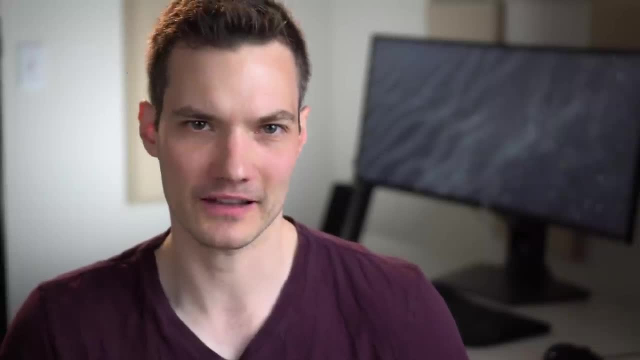 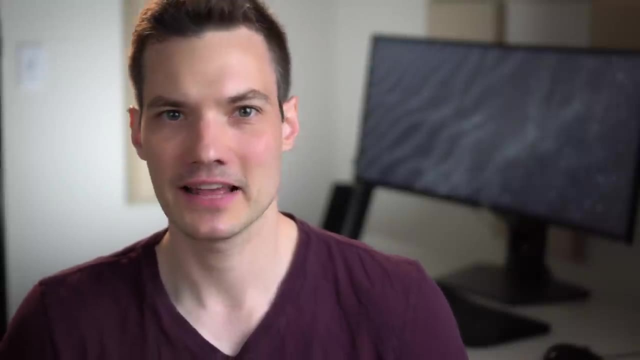 branch to work on that new feature. Maybe someone else is working on a bug fix and they'll create another branch to work on that bug fix And once they finish all of their work and they're satisfied with how it looks, they can merge that back into main Here in File Explorer. 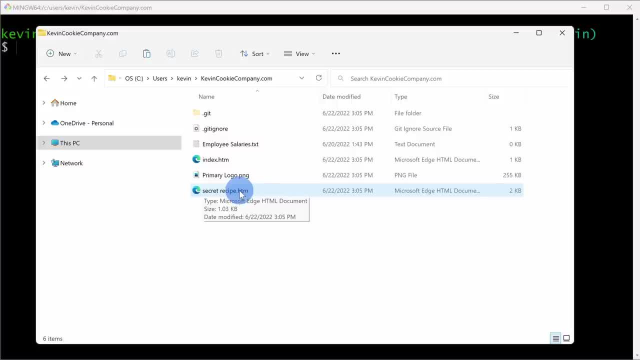 there's a secret recipe and this has the Kevin Cookie Company secret recipe in it. Now I probably shouldn't be showing you this, but we've been working a bit together now and I trust you Let's click into this file Here within the secret recipe. all of this looks pretty good. 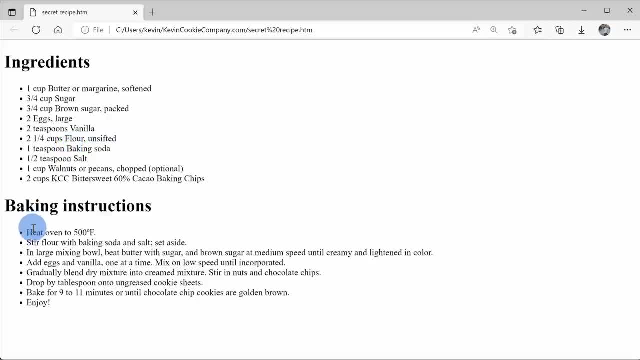 and this is a really good chocolate chip cookie recipe. but right down here I see that it calls out heating the oven to 500 degrees Fahrenheit. That's extremely hot and that would probably work. I need to change this to 375 degrees Fahrenheit. Let's create another branch to. 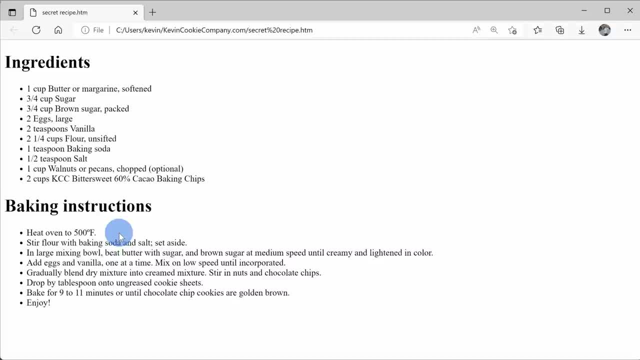 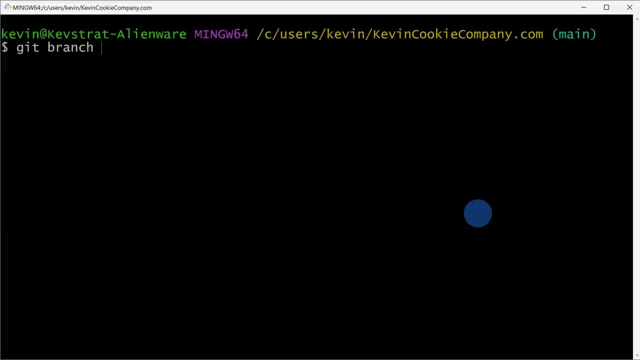 make this change and once we're satisfied with the change, then we can merge it back onto the main branch. To create a new branch, I'll type in git branch and now I could type in a name for this new branch. I want to update or fix the temperature. I'll type in fix temp. 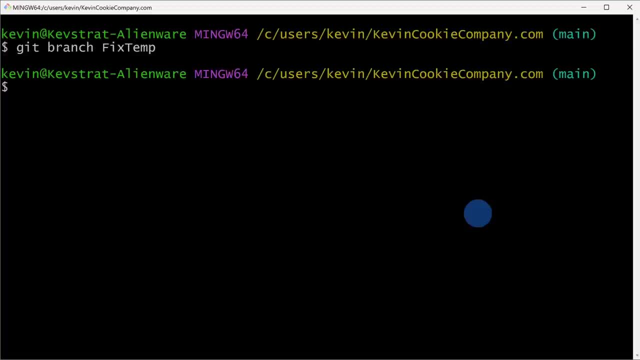 and then press enter. So now we should have two branches. To confirm how many branches we have, I can type in git branch and then hit enter, and here I can see that there's one branch called fix temp and there's another branch that we're currently in called main. How? 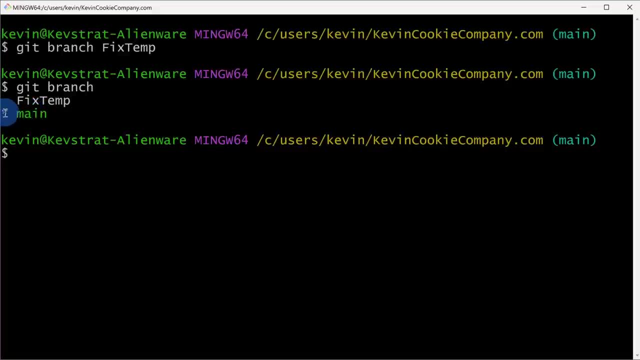 do? I know that we're currently in main. Well, right over here I see an asterisk next to main indicating that this is the currently active branch. To switch into the other branch, let's type in git switch and then I can type in fix temp and hit enter. 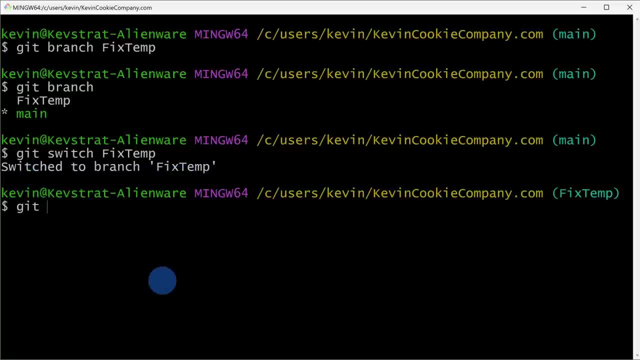 and here it says that we've switched to branch fix temp. Once again I can type in git branch and then hit enter, and here I see that fix temp is the currently active branch, and here I see the asterisk indicating that I've opened up File Explorer and all of the files. 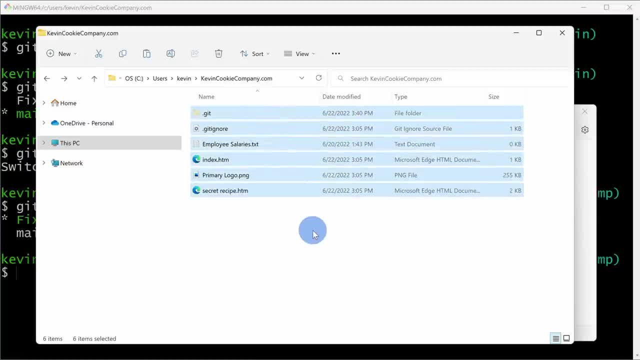 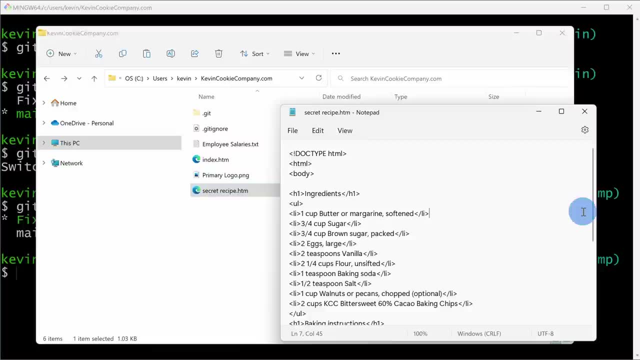 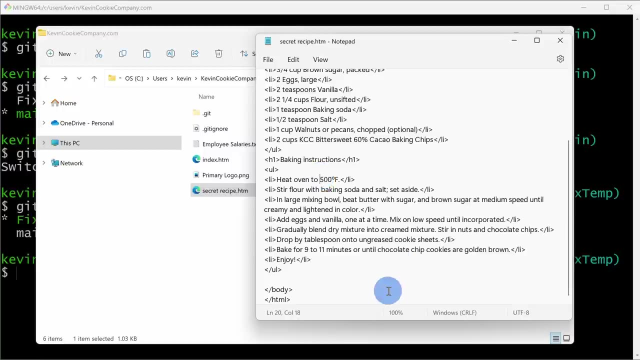 that you see here in the repository. these reflect the fix temp branch. Now I want to edit the secret recipe temperature. I'll take this file and I'll drag it over into Notepad and here I can see the contents of secret recipe. Now, once again, I want to change the temperature down here Currently. 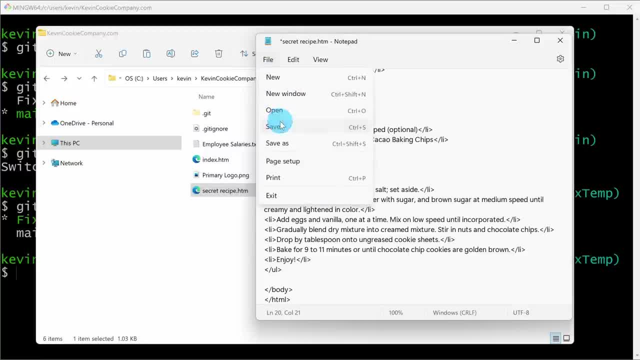 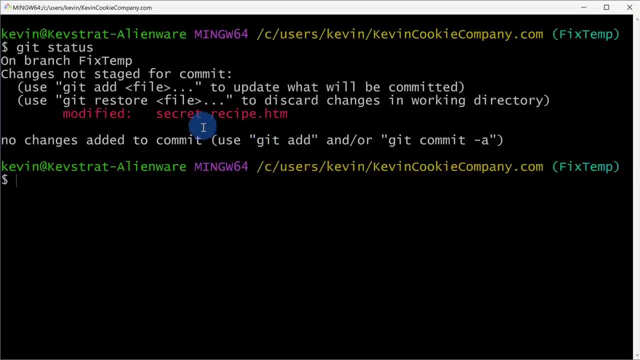 it's 300.. Let's change that to 375, and then click on save. Back now within git bash, let's check the status of this branch. I'll type in git status and then hit enter, and here I can see. 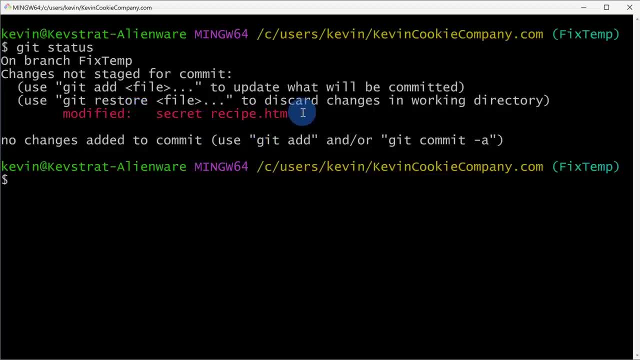 that there is one modified file for secret recipe. We just updated the temperature, so that makes sense. Now I want to commit this change to this branch, Just like we did before. let's type in git: commit dash a, dash m, and then here I'll say: updated temp. 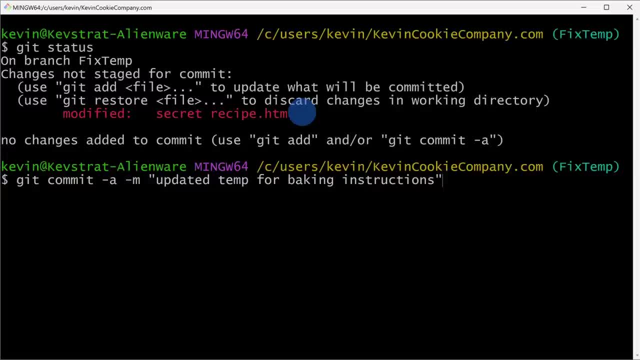 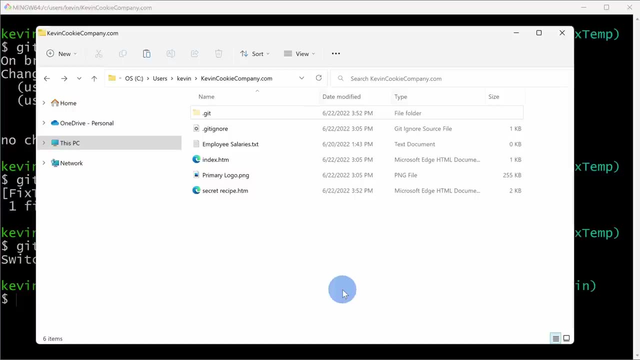 for baking instructions. Then I'll close the quotes and hit enter. and that has now committed the change to this branch. Next let's switch back to main. Here I'll type in git switch main, then hit enter Here within File Explorer, because we switched back into main all of these files. 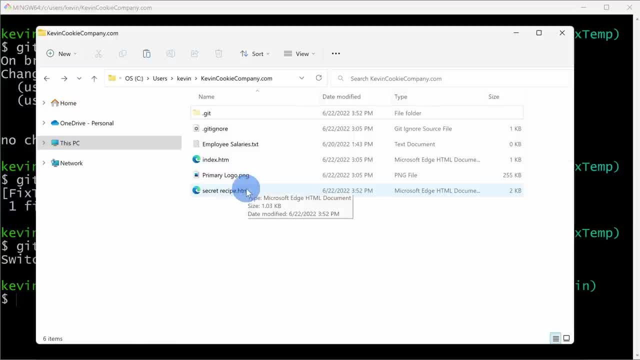 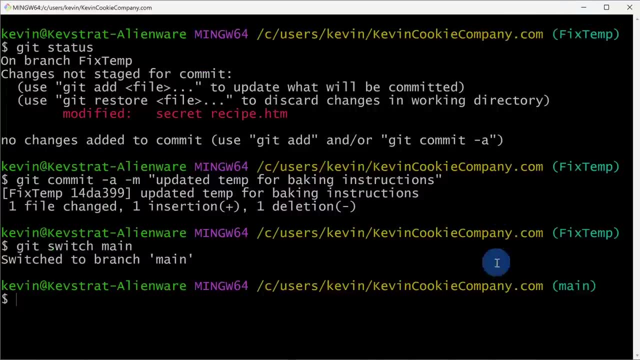 reflect the current state within the main branch. Here, if I click into secret recipe here, we'll change it in the fixed temp branch. We now need to bring those changes from fixed temp back into main or essentially we need to merge those changes in, To merge all of the changes back in. 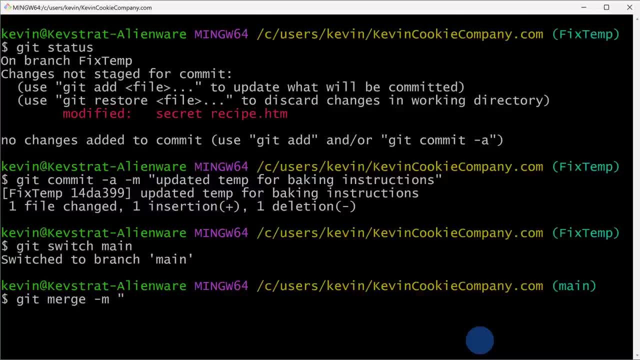 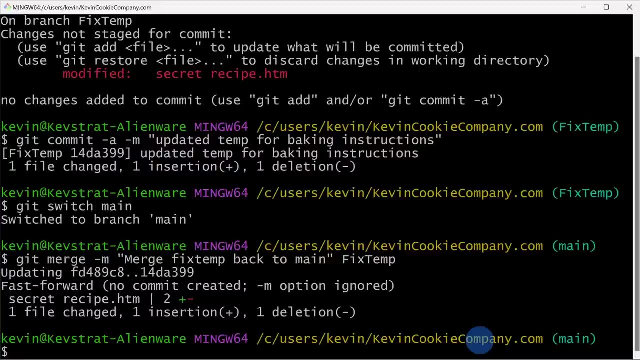 let's type in git merge dash m and here we could type in a message for this merge. I'll type in merge fixed temp back to main and then close my quotes. Then I also need to specify what branch I want to merge back into main. Here I'll type in fixed temp and then hit enter. 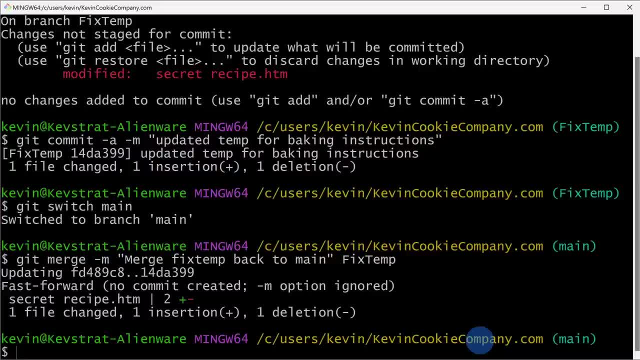 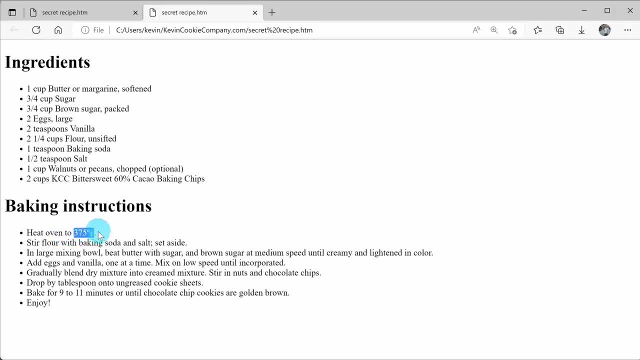 And there I can see that the file has now been merged back into main. Here in File Explorer in the main view I can now click on the secret recipe and here I can see that the change has been merged in and here main is now referring to 375 degrees Fahrenheit for the oven temperature. 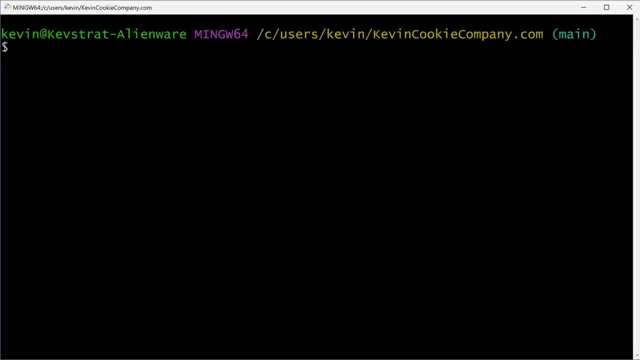 Now that we've merged all of the changes from fixed temp back into main, we no longer have any need for that additional branch and at this point we can simply delete that branch. To delete a branch, Let's type in git branch, then enter dash d, and then you could type in the branch name that you. 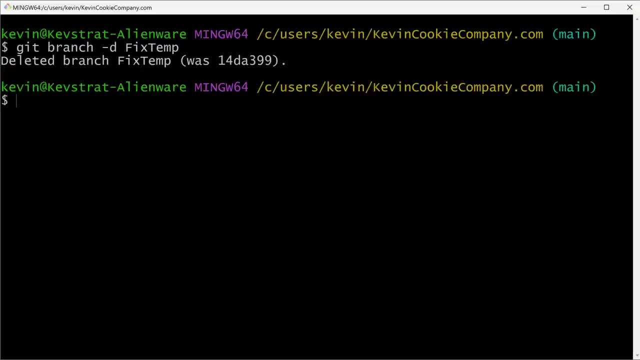 want to delete. I'll type in fixed temp and then hit enter, and that branch has now been deleted. Let's type in git branch, and here I can see that I only have one branch left, and that's the main branch, and that's also the branch that we are currently in. Overall, this merge went pretty. 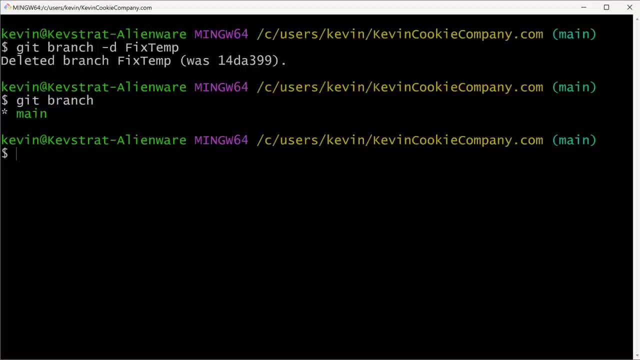 smoothly. Nothing had changed in main, so it was really easy to bring our changes back in. But what if you create a branch and then you try to merge it back in, but main has changed since you created your branch? In that case you'll have a merge conflict. So let's see how. 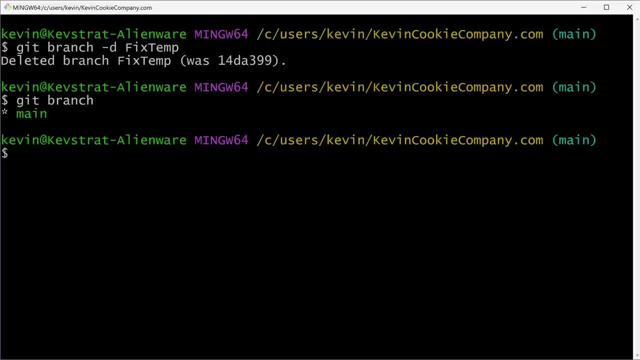 that works, and first let's create another branch. Here I'm going to use a command that not only switches me to the new branch, but it also creates the new branch. I'll type in git switch, dash c. The c will create the new branch, and let's call this one update text and then hit enter. 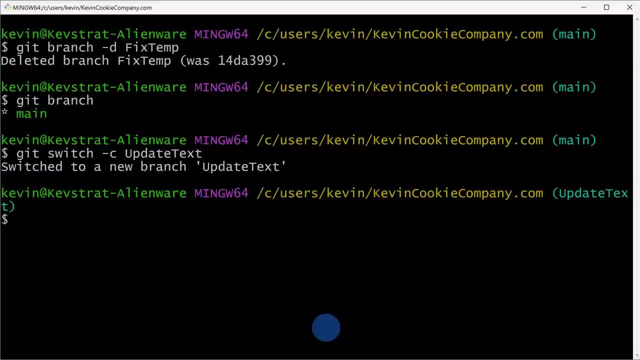 Once again to confirm that we have in fact switched to a new branch. I can type in git branch and then hit enter, and here, once again, I can see that we have two separate branches and we're currently in the update text branch Here in file explorer. once again, all of the 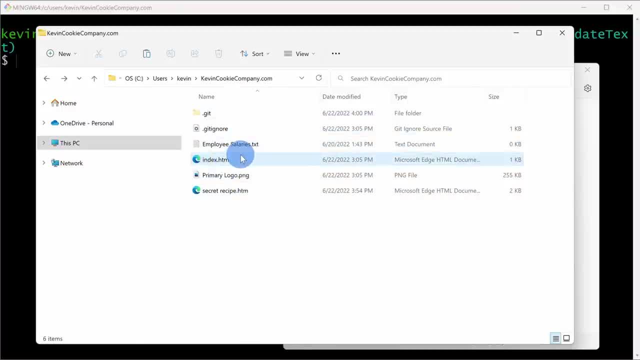 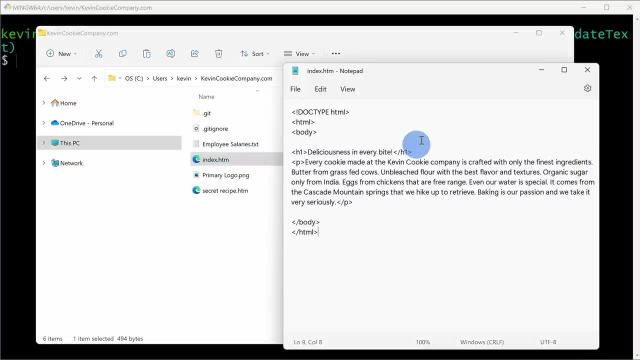 files that you see here reflect the update text branch. I want to make some edits to the indexhtm file. Here I'll take the file and I'll drag it into notepad so I can make some tweaks to it. Here we refer to the file and I'll drag it into notepad so I can make some tweaks to it. 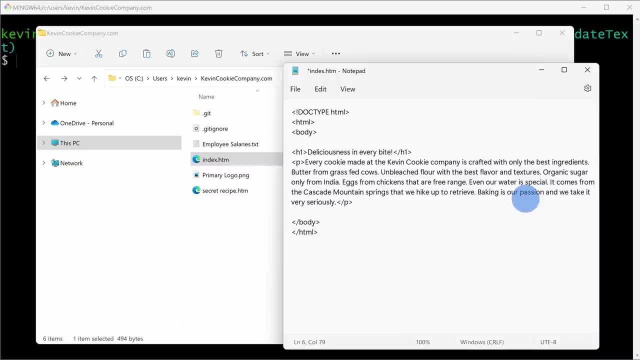 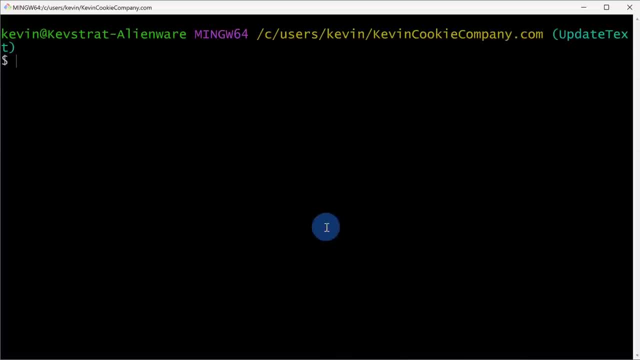 Here I'll save the indexhtm file and back within git bash. let's now commit these changes. Here I'll type in git commit and then I'll type in dash a, dash m, and here I'll say update index text and then hit enter. Let's now switch into main and we'll make a change there as well. 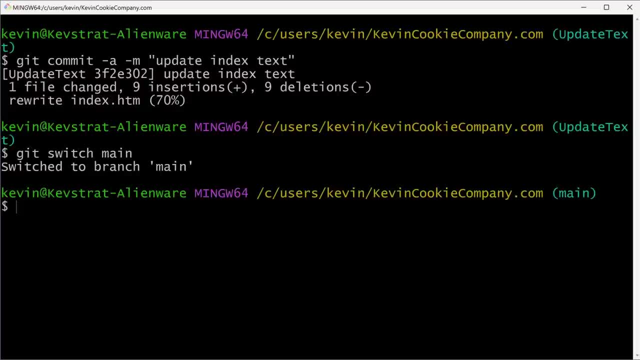 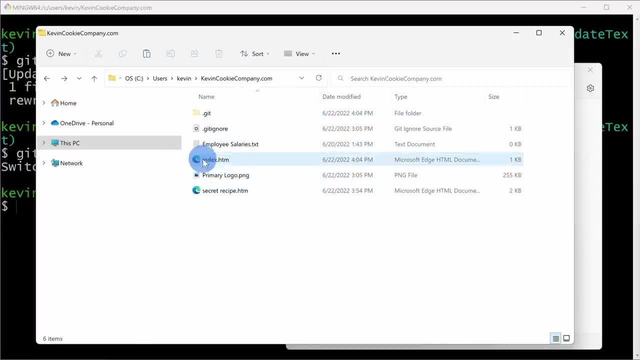 Here I'll type in git switch main and then hit enter Here in file explorer. this now represents the main view, and here I want to make a similar change to the indexhtm file. Here I'll select the file and I'll drag it over to notepad. 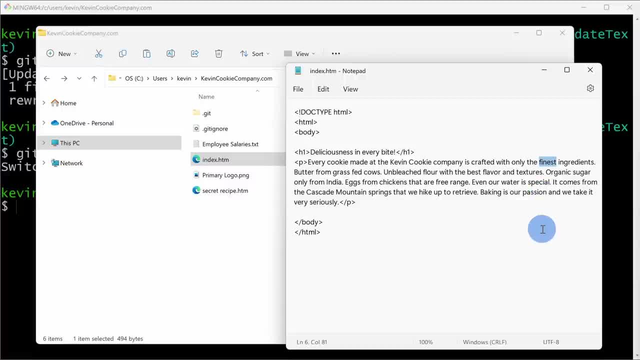 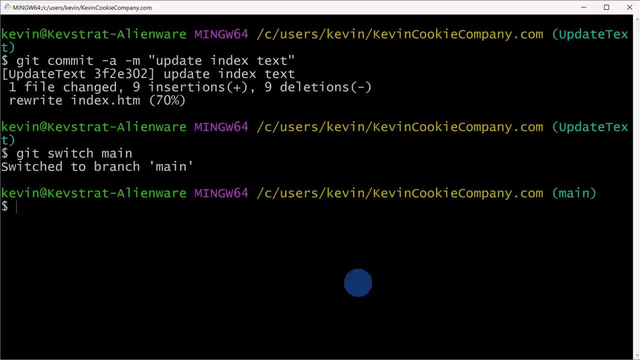 and here it refers to the finest ingredients, Let's say maybe the most amazing ingredients, and then I'll save this file and close it Back now in git bash, let's commit these changes to main. I'll type in: git commit dash a. 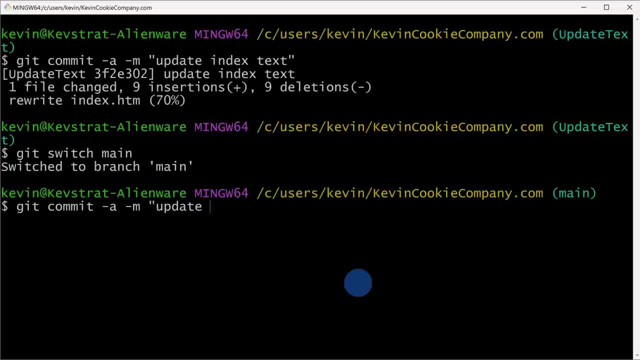 and then dash m, and here once again I'll make some changes to it. Here once again I'll say update index text and then I'll hit enter. So I've now committed this change to main. Let's now try merging the changes from update text back to main, to. 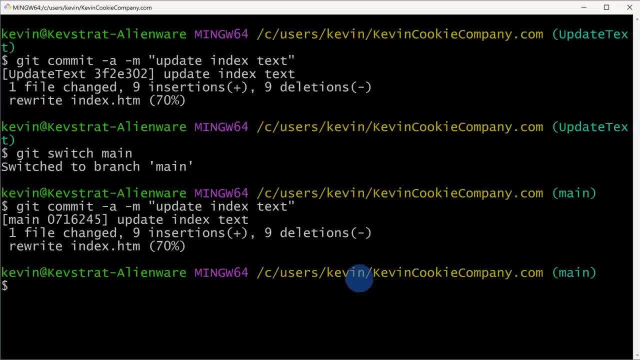 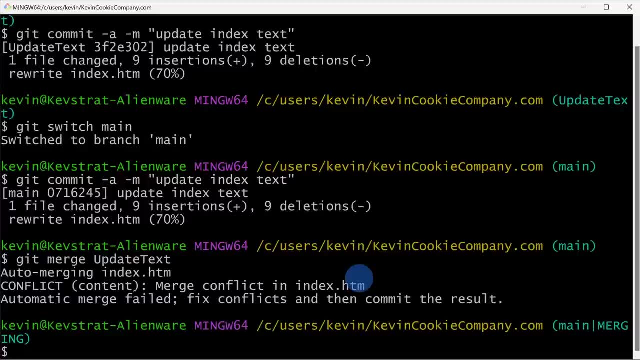 see what happens To merge, update text to main. let's type in git merge and then update text. and let's see what happens when we press enter. When I press enter here, I get an error message telling me that the merge failed and the reason why is that there are conflicts And right down. 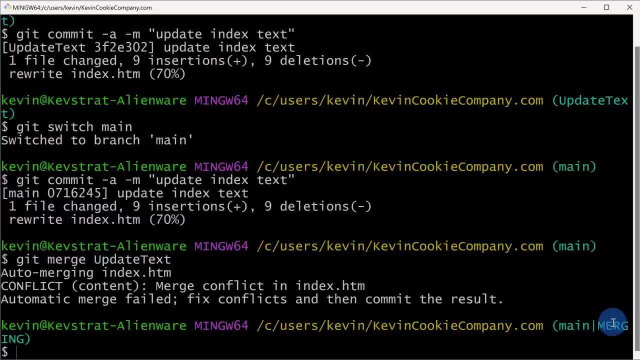 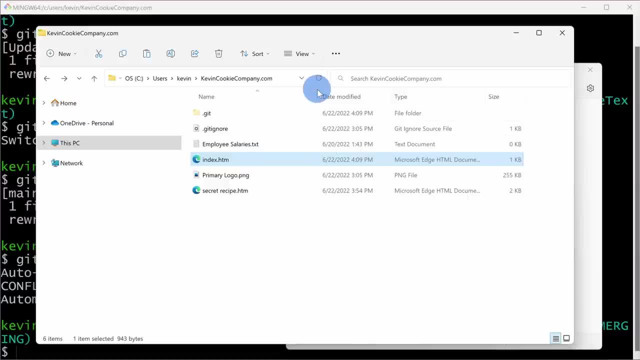 the bottom right hand corner, I can see that I'm currently in a branch called main merging. Let's go back to file explorer to see if I can resolve these merge conflicts. Here in file explorer I can see all of the files for the merging view and, if you remember, we had a merge conflict with 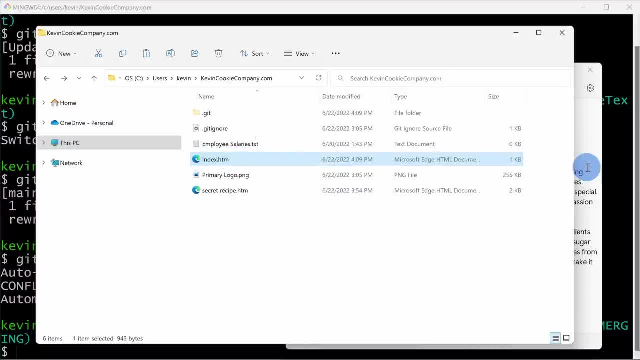 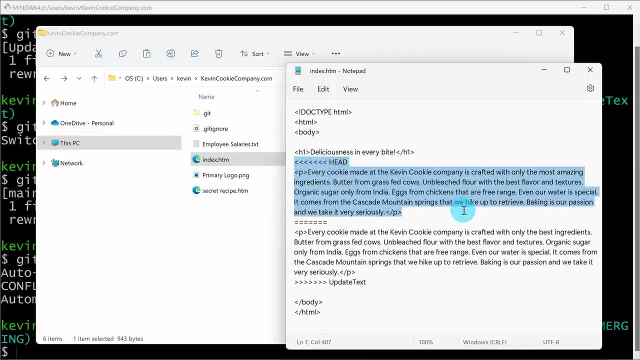 the indexhtm file Here. I'll drag that file into notepad and here I can see some text that says head. Head refers to what's the current reality or what's currently in main, and down below I can see that I'm trying to bring in from the branch update text and I can decide which one I want to. 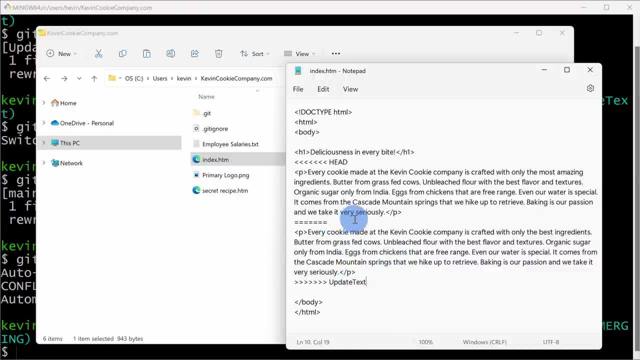 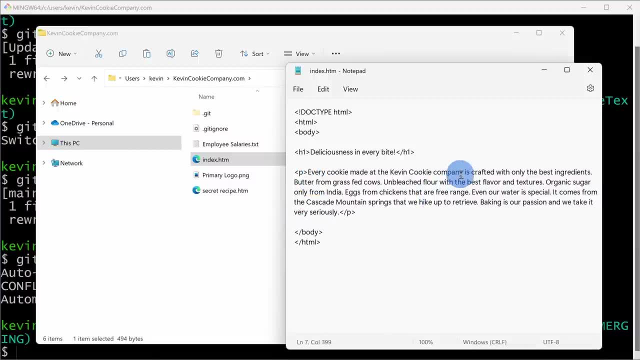 keep. Now I want to keep the text from update text. so here I'll delete the head and here I'll delete this portion and then I'll save the file. Let's go back to git bash. Back in git bash. 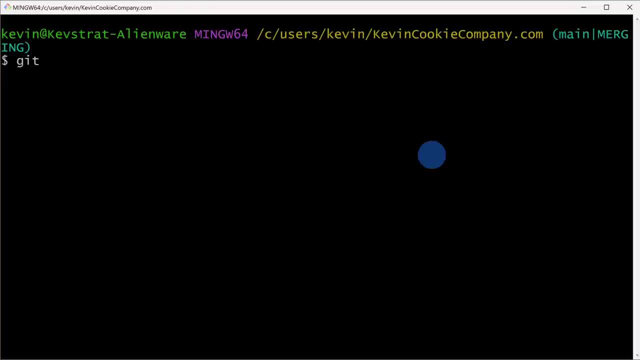 I can now commit the change Just like we've done before. I can type in git: commit dash a, dash m and then update text on index and then I can close my quotes and hit enter and that's now updated, that merge conflict. That's one way you can resolve your merge conflicts. 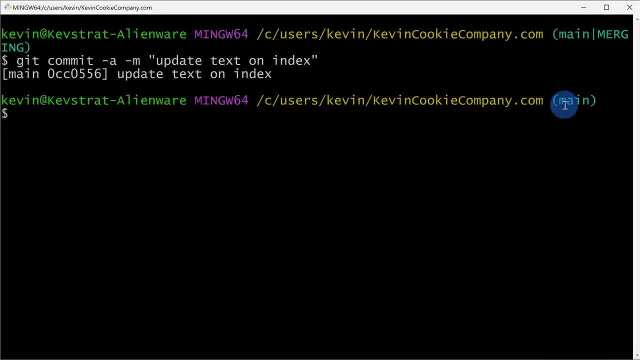 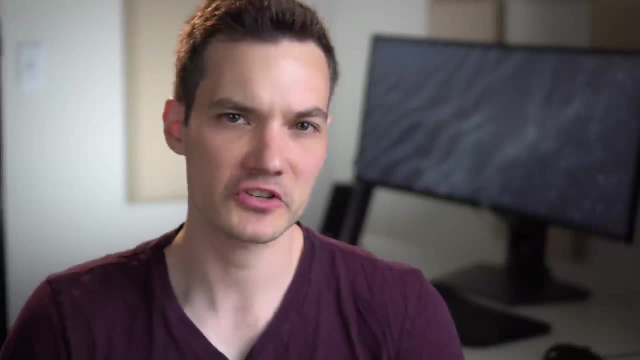 and now that I've resolved that conflict here, I can see that I am now back in main. This should give you an idea of the typical flow that most people use in git. You have some feature or bug that you need to work on. First you'll create another branch, then you'll go in and 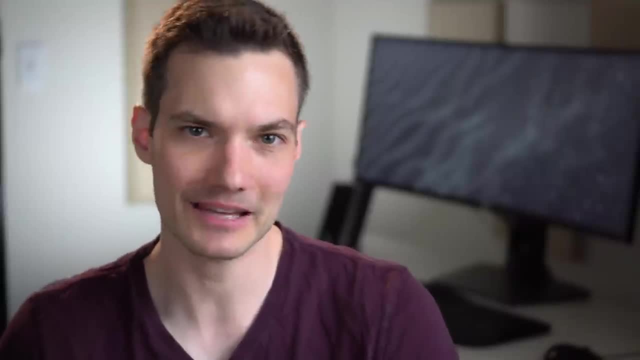 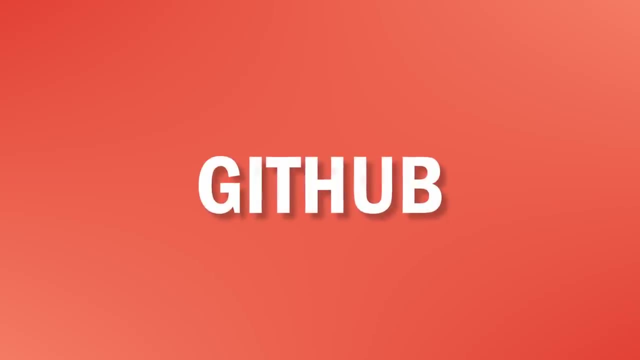 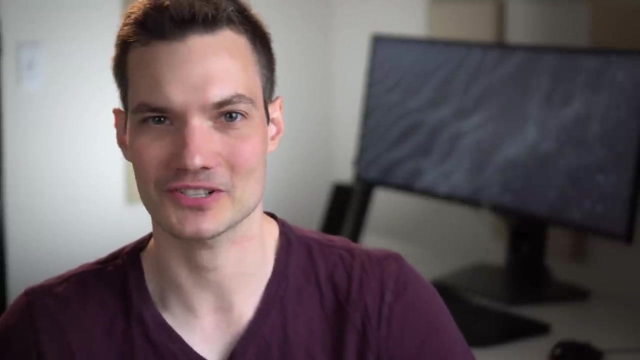 you'll make all of your changes. then you can merge it back into the main branch and once you are working on, Now that you understand the fundamentals of working with git, you might be wondering: well, how do you work together and collaborate with others? So far, we've just been 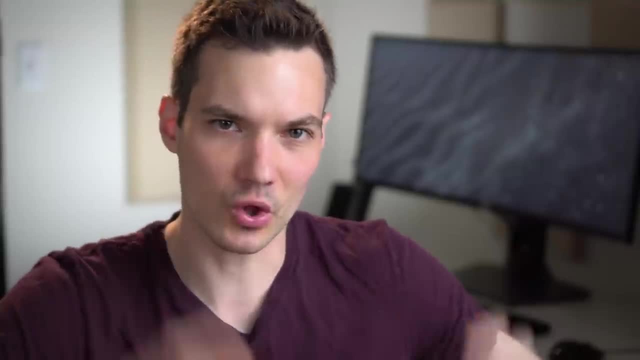 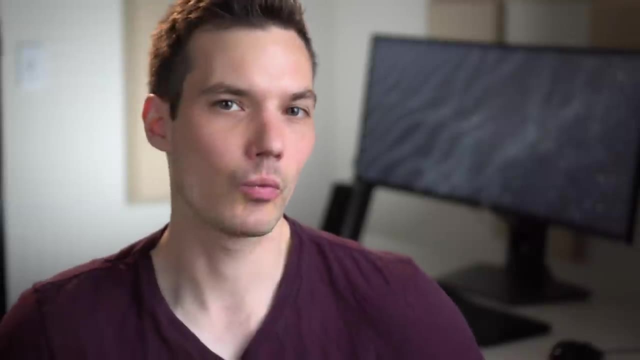 working with a git repository that's hosted on your local computer, but you can also host your git repository in the cloud, and one of the most popular cloud repositories is called GitHub. Not only do they offer a cloud-based repository, but they also offer a cloud-based repository for your. 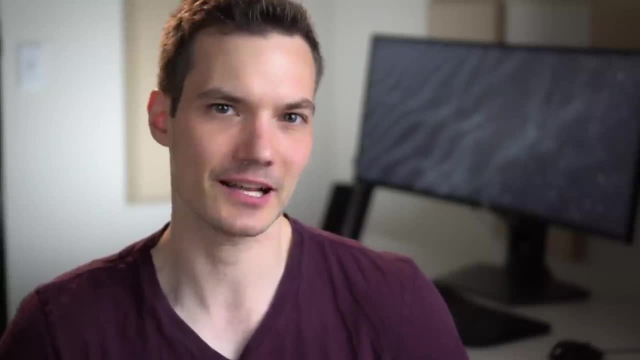 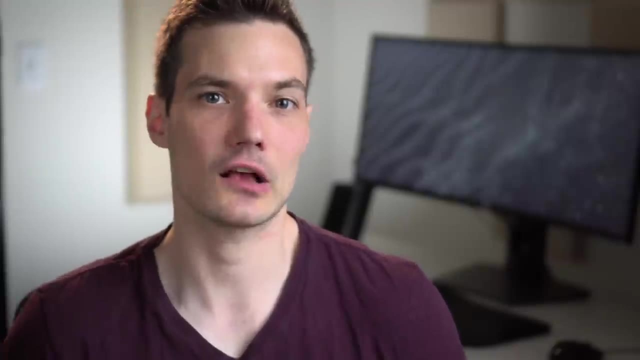 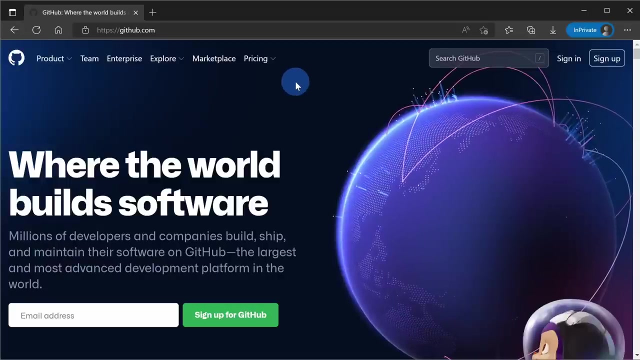 cloud repository, but you could also manage your project. You could set up Kanban boards, you could track issues, you could assign features or bugs to different people. In a sense, it's a social coding website. Let's check out how you can get started with GitHub. First, we need to 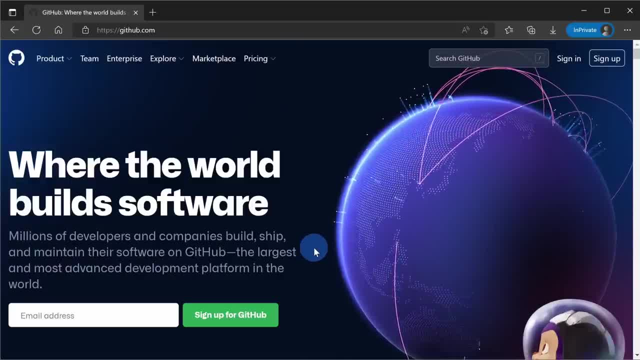 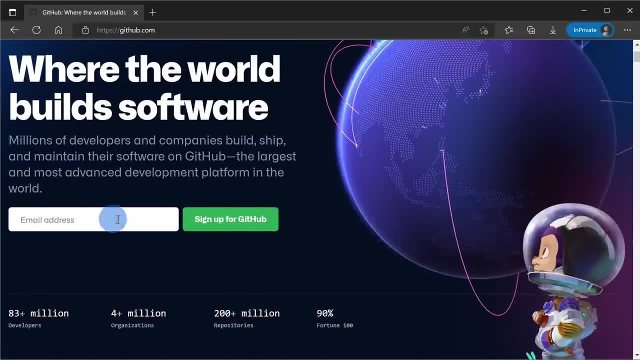 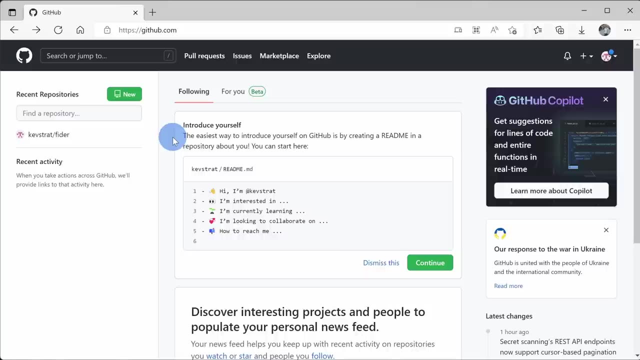 create a GitHub account, You could head to the following website. You could click on a link up above or also down below in the description On the homepage type in your email address to kick off the flow for creating a new account. Once you finish setting up a new account, we can now create a cloud repo. 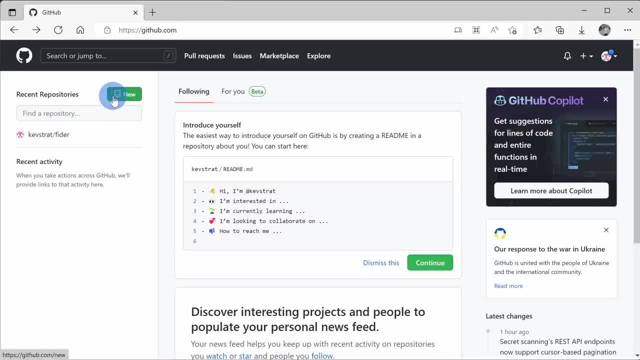 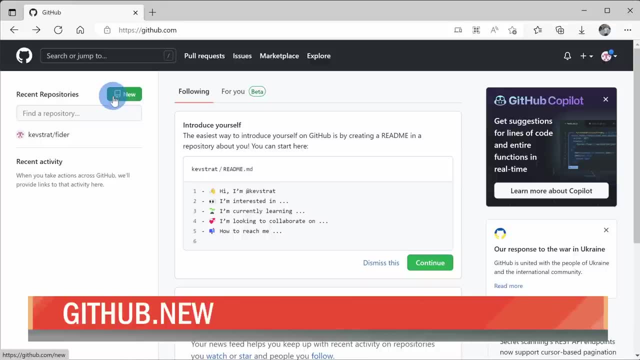 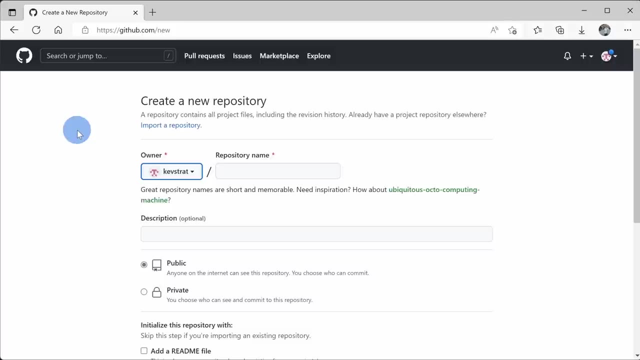 Over on the left-hand side, you should see the option to create a new repo. Alternatively, you can also head to the URL githubnew and that'll also drop you on the new repo page. Let's click on this. You might be wondering: do I really need to create a cloud repo, especially if 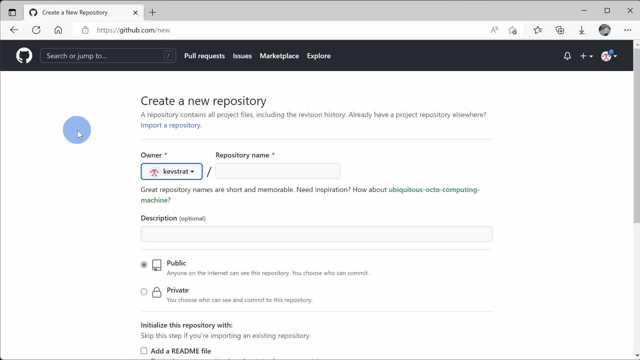 you just plan on working by yourself. Well, if you're planning on working with a team, it makes really simple. Open up the local cloud repo so you can all work together. But even if you plan on just working by yourself, by storing it in the cloud if something happens to your local computer. 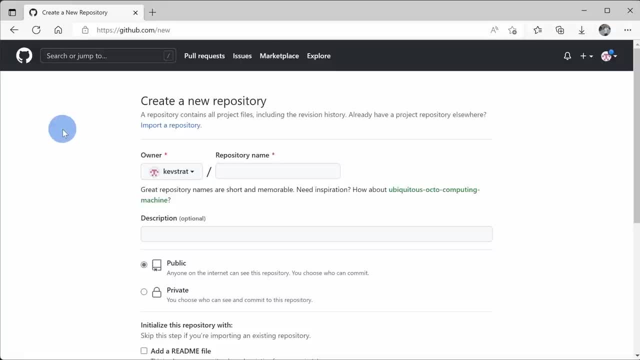 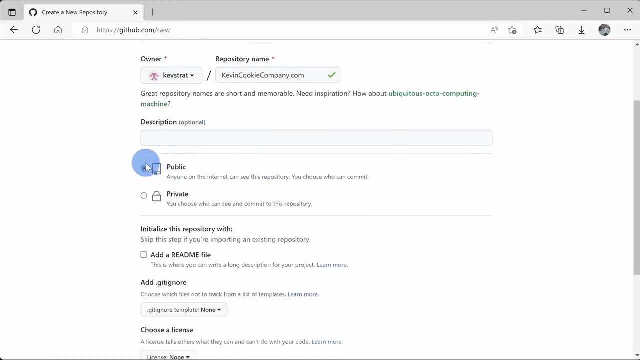 you have a backup and all of your repo files are safe. To set up a new repo over here, I need to enter in a name for this repo. I'll type in kevinkookiecompanycom Down below. I could also type in a description for this repo. I'll leave it blank for now. Here I could decide. do I want to? 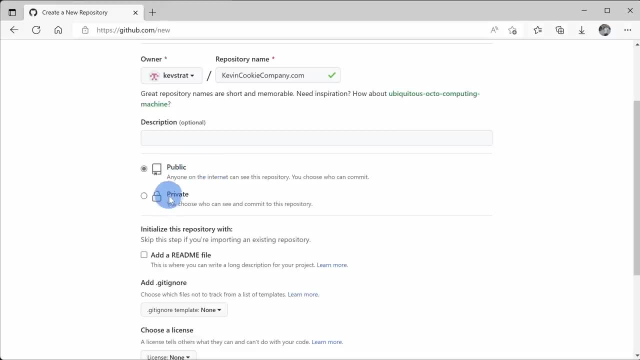 this repo public so anyone can come in and access it, or do I want to make it private? If I make it private, I could assign different individuals access to my repo, so I could just work with a smaller group of people Down below. I also have some other options Here. 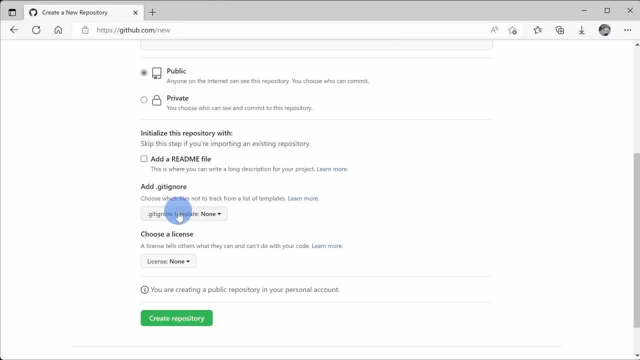 I could add a README file. I could also add a gitignore file. Remember earlier, when we were working with our repo, we manually created a gitignore file, but here you could just create one as you create your repo, and down below you could also choose to add a license. Now, 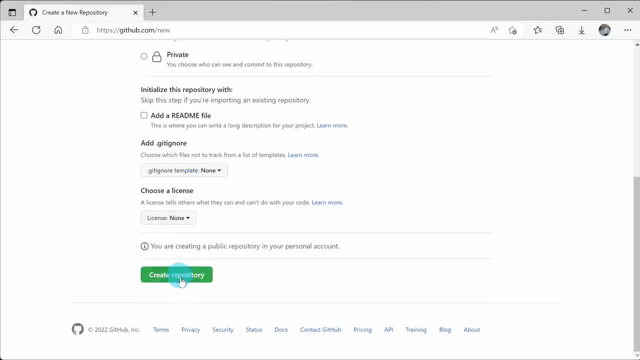 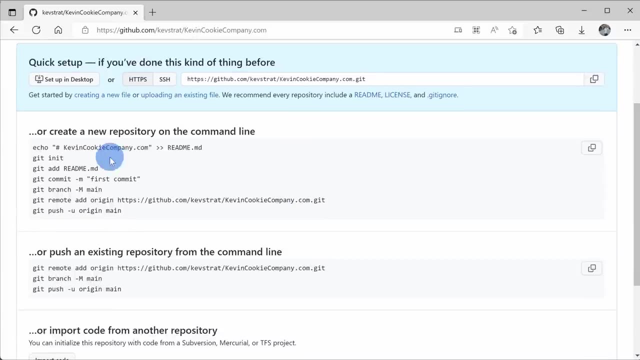 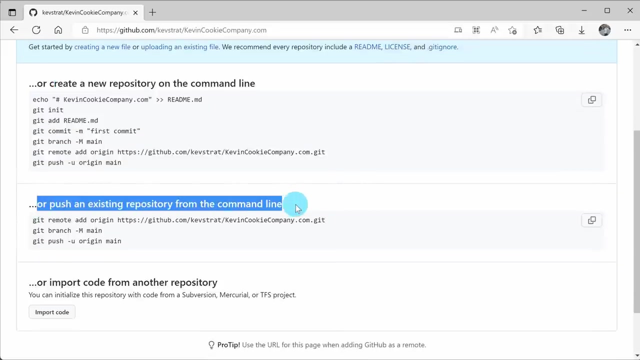 all of this looks good, Let's click on create repository. Now that we've finished creating our repository, here I see a quick setup guide. Right here I can see how to create a new repository on the command line. Right here I see the option to push an existing repository. 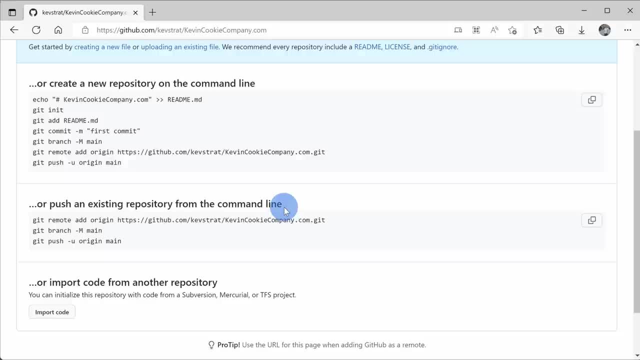 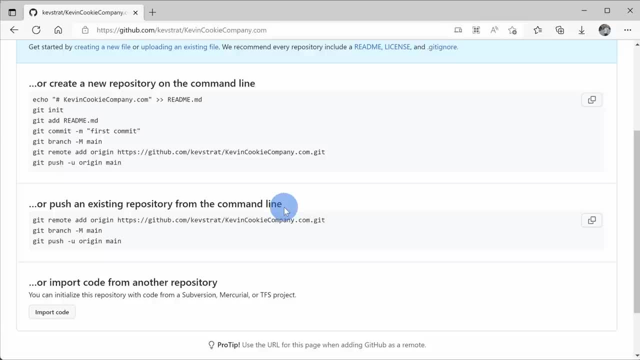 on our local computer that we can create on our local computer that we've been working with for most of this video. We can take that repository and we can push it into the cloud. So let's take this first command, git remote- add origin, and then this URL: Your URL will: 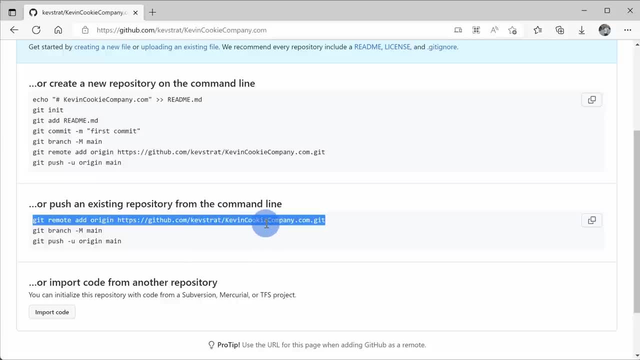 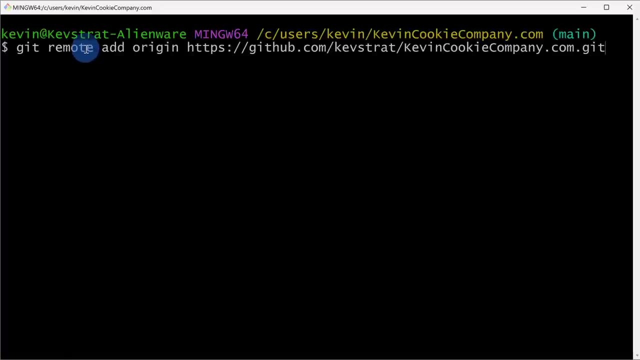 be specific to your GitHub account. Let's copy this and then go back to Git Bash Within Git Bash. here you could right click and you could paste, or you could press shift and insert to paste what we just copied Right here. this is establishing a remote connection with GitHub and we're calling 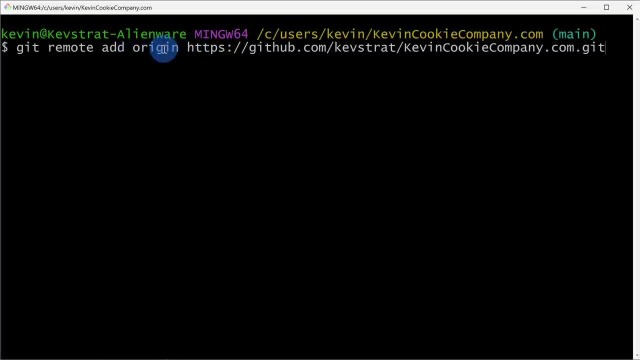 this remote connection origin. That's a common name that most people end up using, and here we can see what the address is that we're going to connect to. Here I'll press enter. Let's now go back to the website to see what the next command is. The next command will set the target branch to. 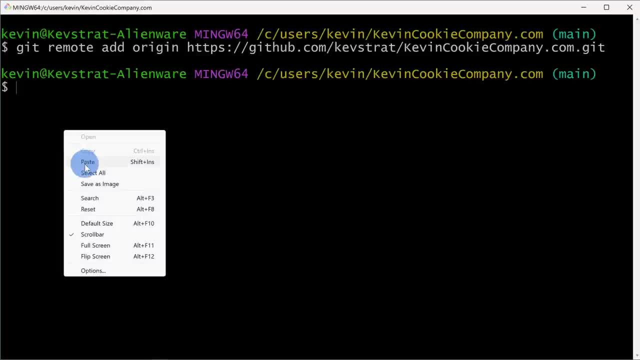 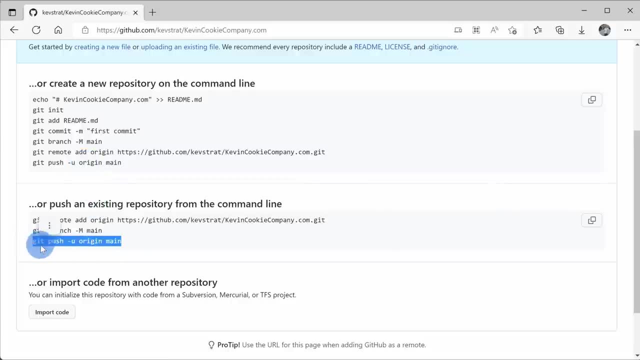 main. Let's copy this and then go back to Git Bash and here I'll paste this in, and then let's run that command as well. Once again, let's go back to GitHub, and here we can now push all the contents. 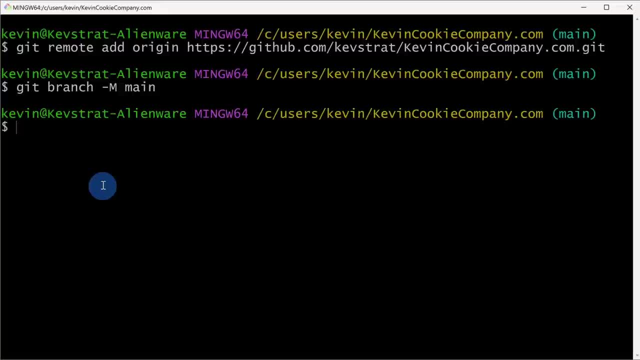 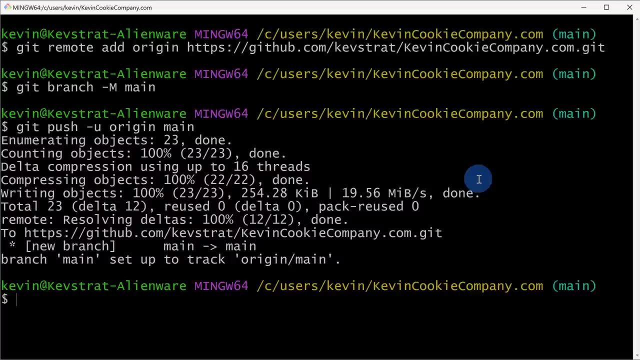 from our local computer to our local computer. Let's go back to GitHub and here we can now push local repository to the cloud. I'll copy this and then let's paste this in and once again let's press enter, and here I could see that my entire local repository has now been pushed. 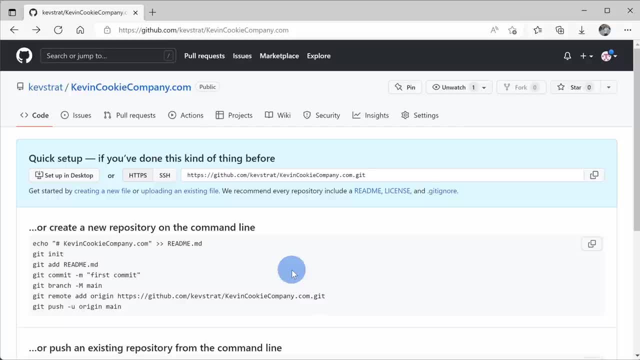 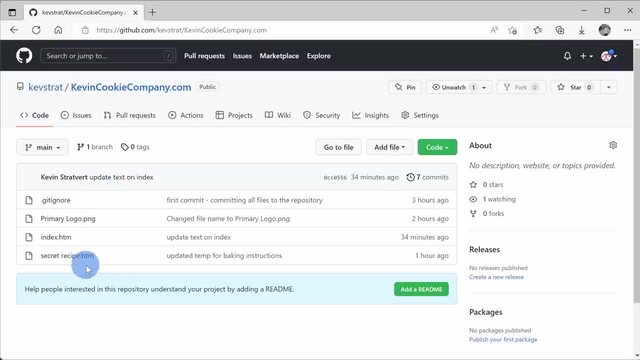 to GitHub into the cloud repository. Back on GitHub. here I could click on the repository name kevincookiecompanycom and check that out. Here I can now see all the files from my repository synced onto GitHub, and that's pretty cool. Right up here I see that there's currently. 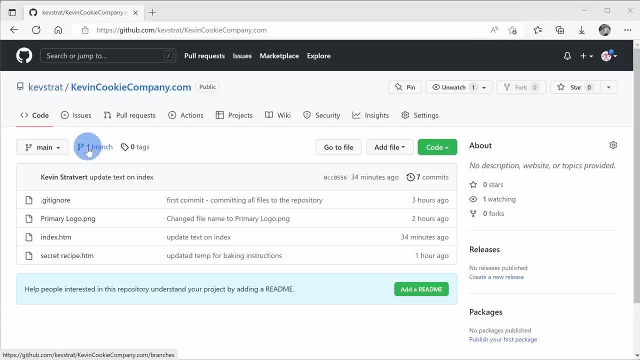 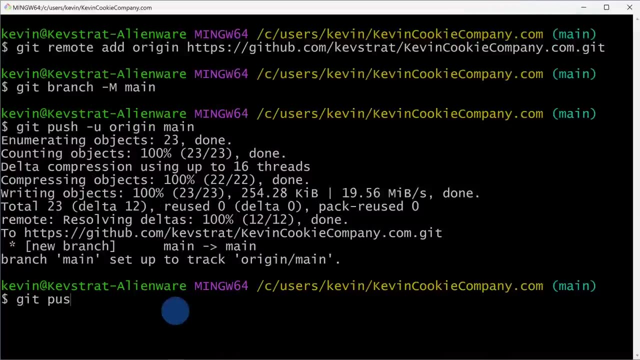 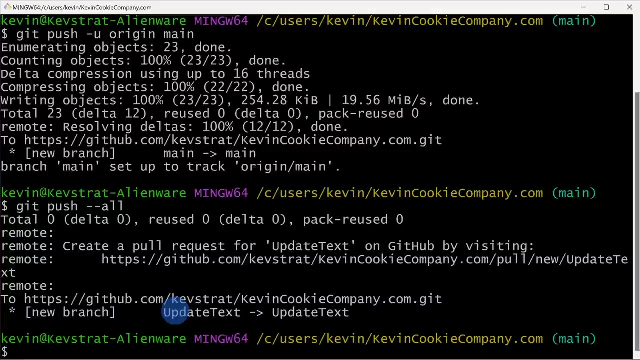 only one branch and I had another branch called update text. If we go back to Git Bash, I could also push through all of my branches Here. I could type in git, push, dash, dash, all, and that'll push through all of my branches to GitHub. Let's press that, and here I can see that it also passed. 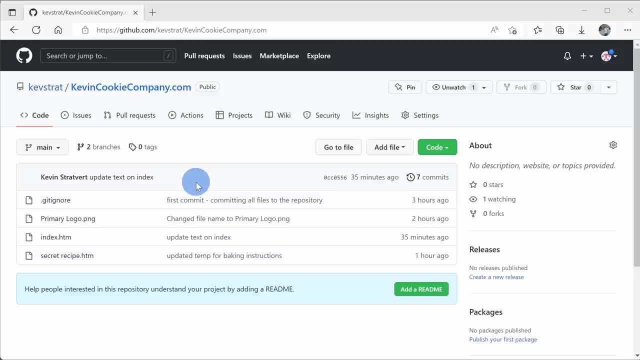 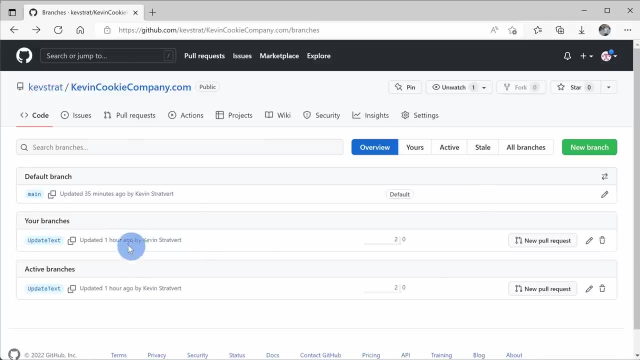 through the update text branch. Let's go back to GitHub. Here within GitHub, I can see now that there are two separate branches. I have my main branch and then I also have the other branch titled update text. Now that we're on GitHub, let's take a look around to see what we could do. 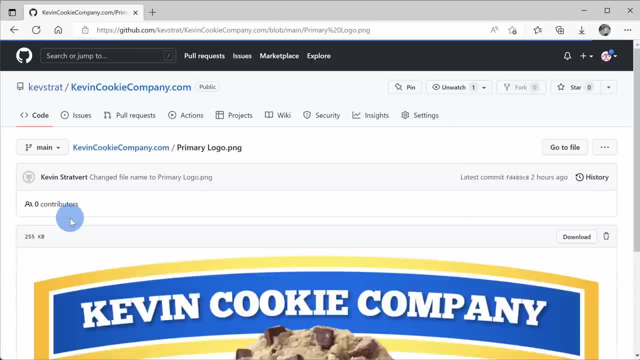 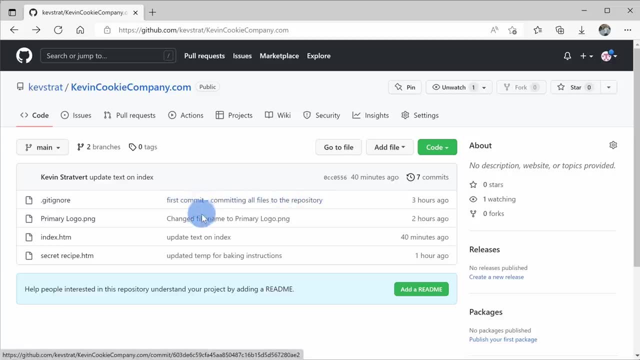 Here I could click on my different files. Let's say I click on my primary logo dot png. Here I can preview what that looks like Here I'll go back Right here. I could also see what the last change or commit was for a specific file. 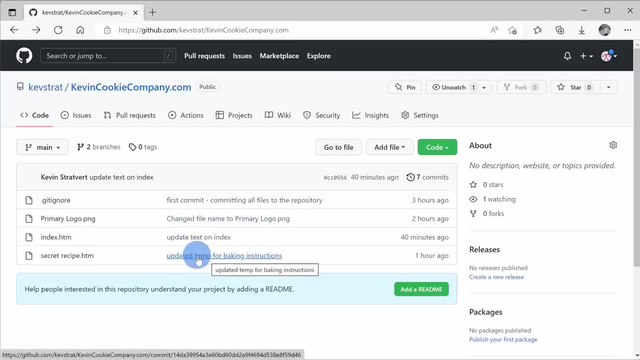 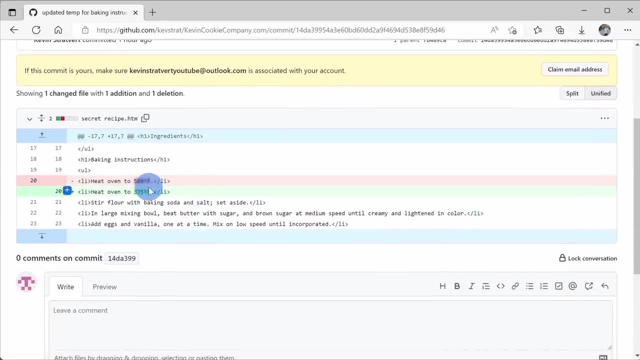 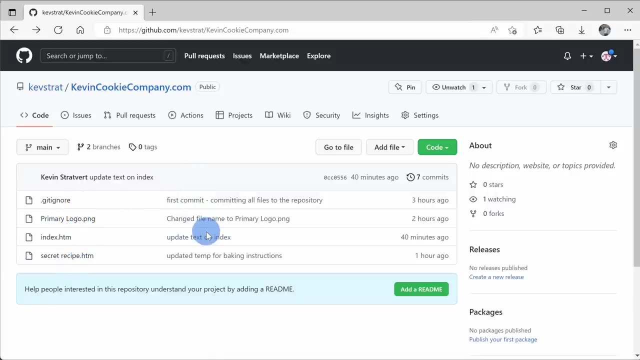 Right here with the secret recipe. here I can see that we updated the temperature for the baking instructions Here. if I click on that, I can review what it was and what it was changed to Back on the main screen. if I want to add additional files here, I could simply drag and. 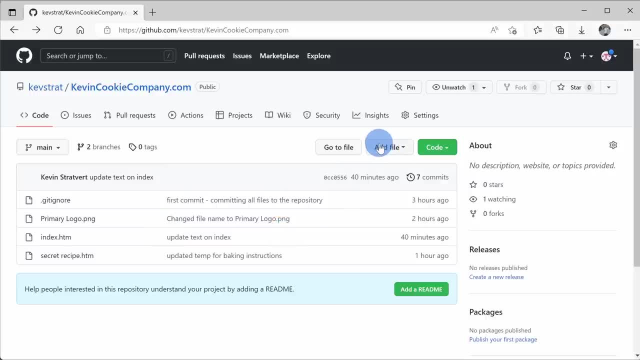 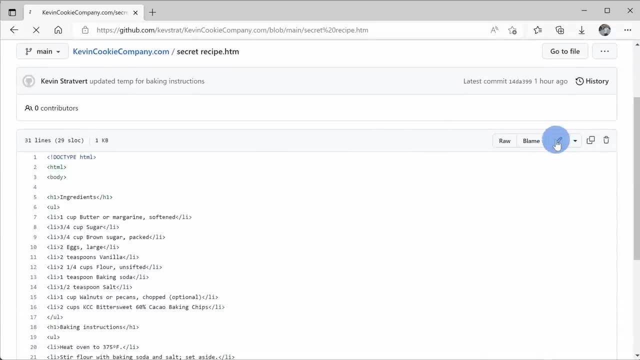 drop them onto GitHub, or I could click on add a file right up here. Let's say I want to edit one of these files. Here I could click on the file name, secret recipe, and here I could click on this edit icon and I could go through and make changes directly in here Once I'm all done. 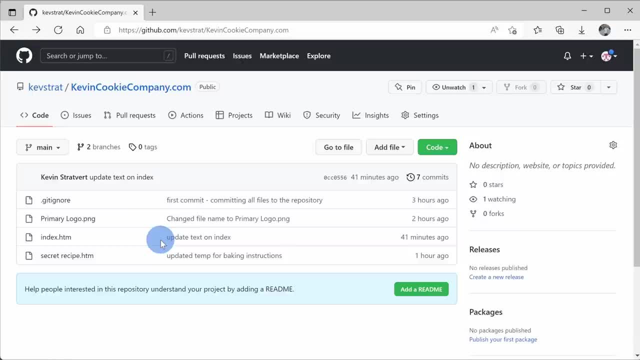 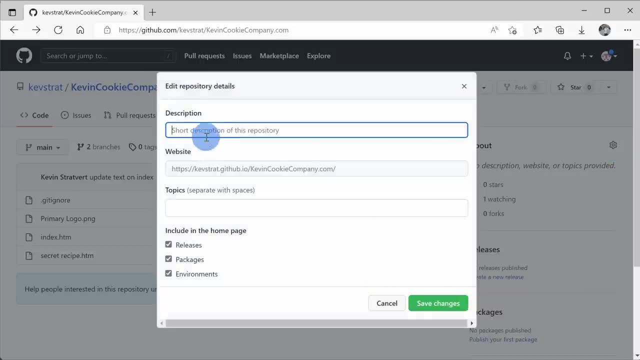 I could also commit directly on GitHub Back on the main repository view over on the right-hand side. here I could edit details about this project. I could click on this settings gear and I could type in a description the website. I could enter various topics and here I could decide whether I 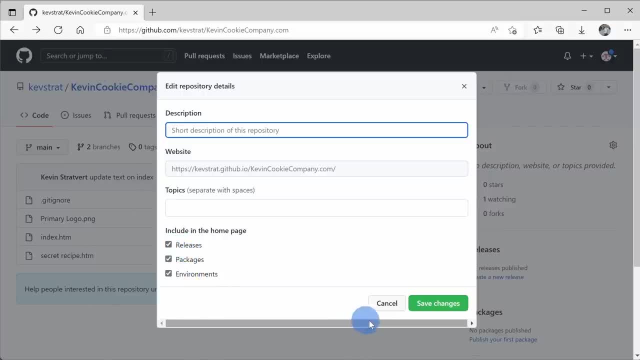 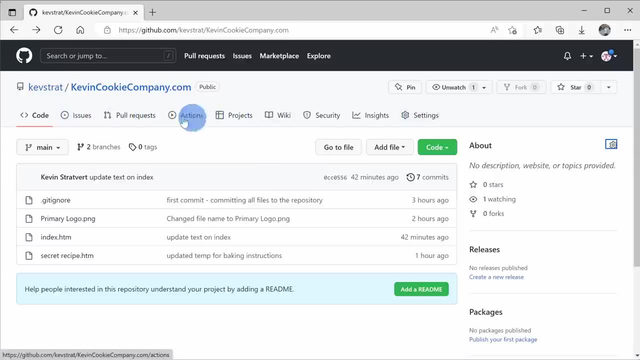 want to include releases, packages or environments directly here on the repository home screen Up across the top of the page, we have all of these different tabs related to the project and the first one is called issues. Let's click into this one. 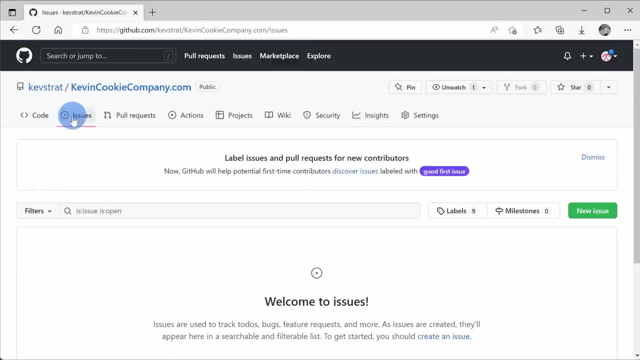 Issues is where you can enter in feature requests, or maybe someone finds a bug. You could enter the details of that directly into this page. So let's say that. on the home page I notice that we say that we get our sugar from India. 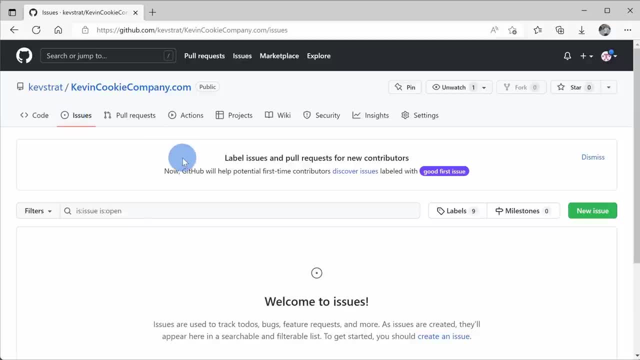 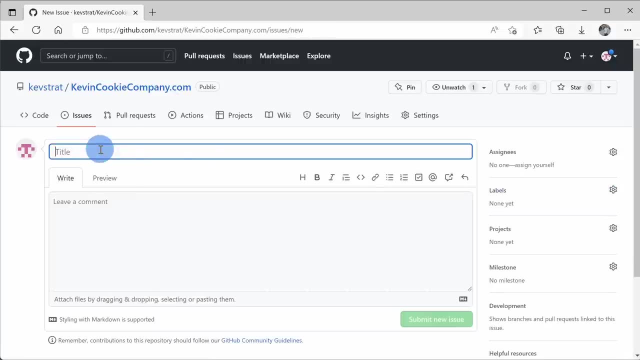 but it turns out we also get it from the Philippines, so that's a bug. on our home page Right over here let's click on new issue. On the issues page over here I can give this issue a title and let me type out we should call out that organic sugar. 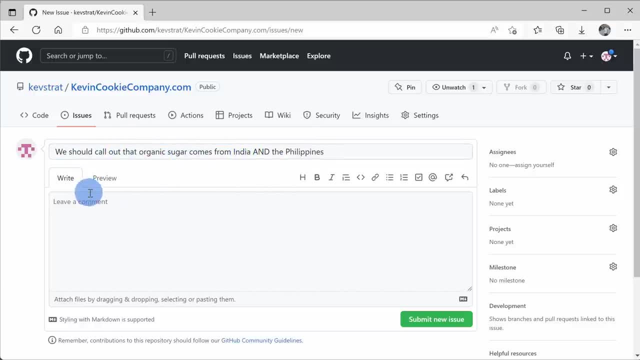 comes from India and the Philippines. Over here I could also type in additional details or comment. Over on the right hand side. I can assign this issue to someone Now. currently there's no one else on my team, so I will assign it to myself, just so I can keep. 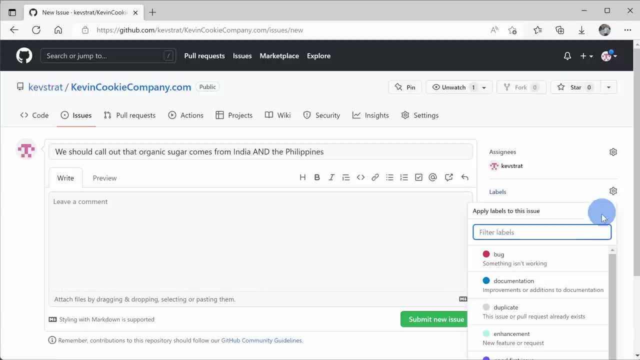 track of this issue Down below. I could also assign a label. I'll click on the settings gear and here I could add a bug. but you have all these other labels as well. I'll select bug Right here. I could also assign it to a project. I could also assign various milestones. 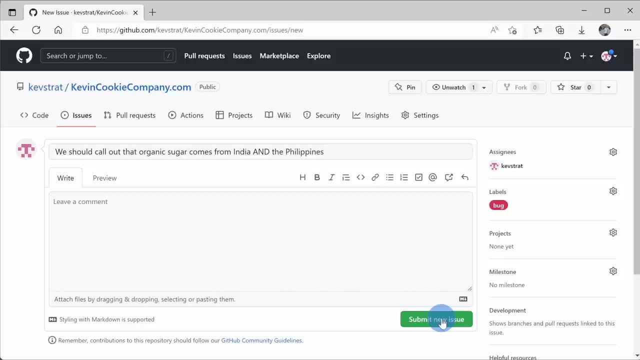 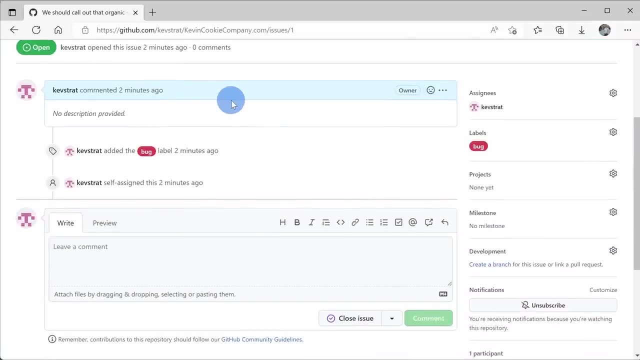 And I'm all done entering in the details here, so let's click on submit new issue. This has now successfully created an issue, and the great thing in GitHub is it's a social environment, so other people could come in here, They could leave a comment, We could discuss. 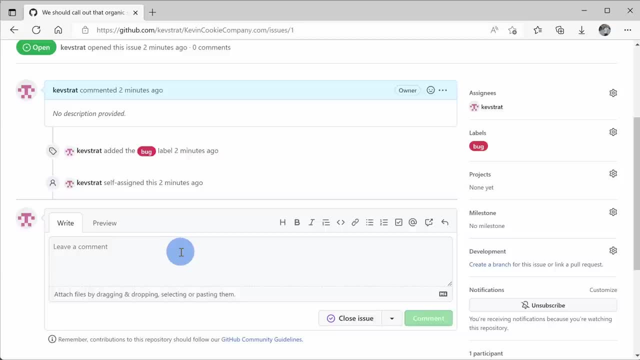 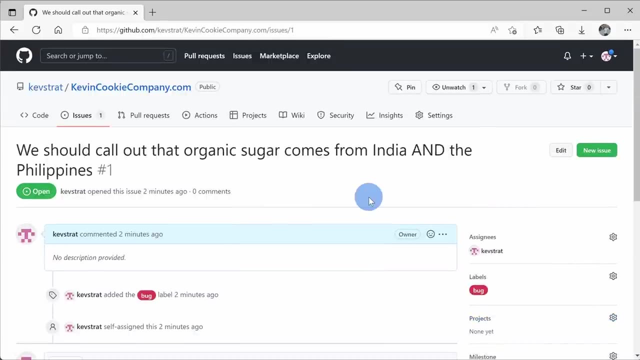 is this truly a bug that needs to be fixed, and maybe what priority should we give it? We could have that discussion all right here within this page. Now I have this issue assigned to myself, so I should probably get to work and update our 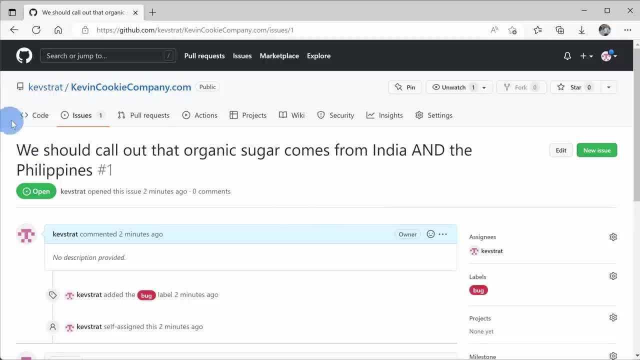 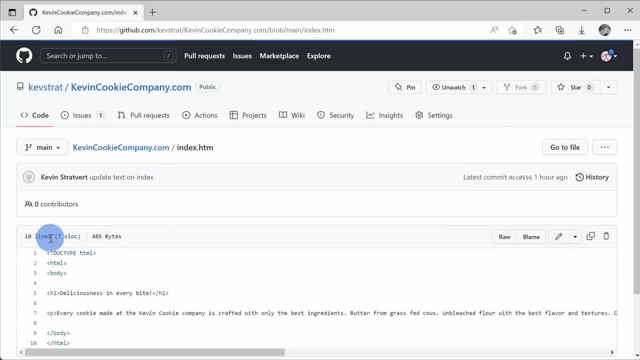 index page to also call out the Philippines. In the top left hand corner, let's click on the code tab. right here I have my index file. I want to edit this. I'll click on indexhtm and over here let's click on this edit icon Within the edit view right up here. 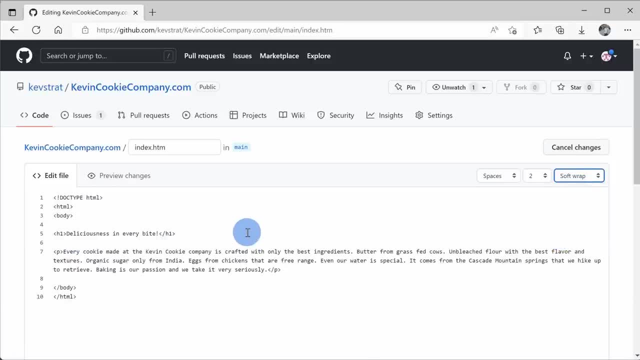 let's change it so it wraps. So here I can see all of the text on this page and if I look right here, it calls out organic sugar only from India, and of course we also get it from the Philippines. So here I'll say: end the Philippines. Now I'm all done making my changes. 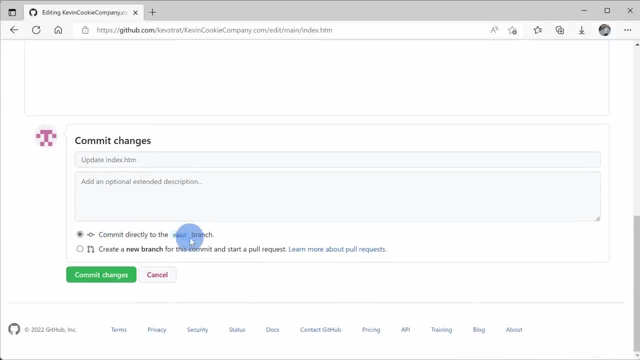 If I scroll down just a little bit, I can see that I've got a lot of changes. If I scroll down just a little bit here, I can commit it directly to the main branch, or I have the option to create a new branch for this commit and to start a pull request. So what is a pull request? Well, I can. 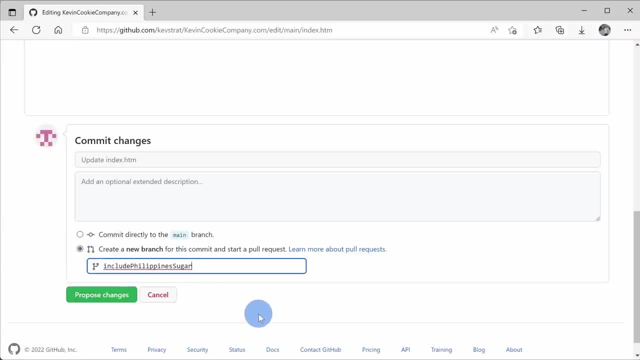 start a new pull request and then this change has to be approved. so, especially if you're working with others, you can have other people go in. they can make changes and then you can have them submit a pull request. so the change has to be reviewed by someone before you push it through. to the main branch. I'll get to that in a minute. Now I'm going to go ahead and click on the pull request. I'll get to that in a minute. I'll click on the pull request Here. I can commit it directly. 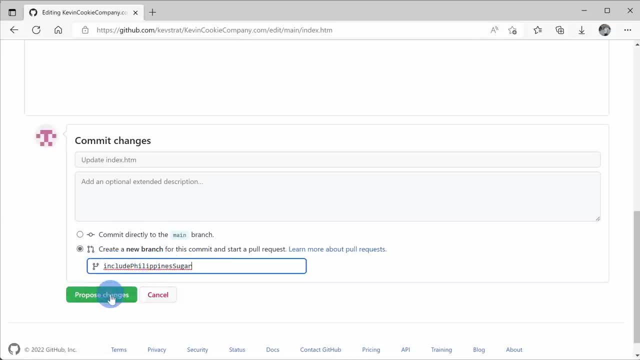 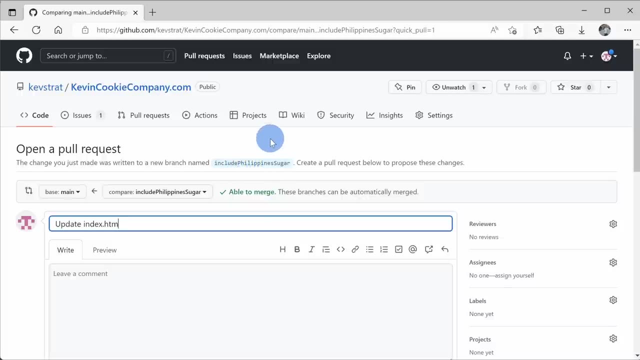 this new branch a name. I'll call it include Philippines sugar and then click on proposed changes. This has now successfully created a new branch called include Philippines sugar, and now I want to submit a pull request. This is basically a request for someone to approve. 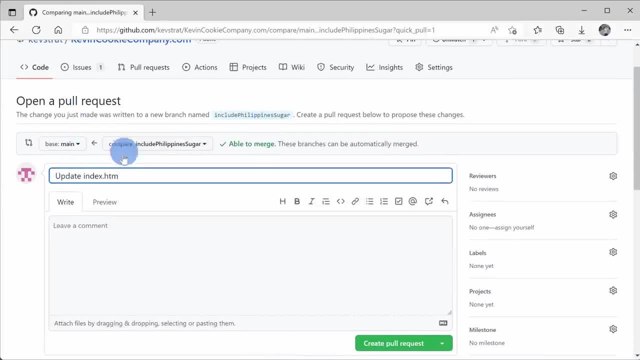 merging this back to main. Right down below I can see the pull request details. It says update indexhtm. but I probably want to be a little bit more explicit. I'll insert a dash and maybe include some text that says we should include Philippines as one of the countries that we get. 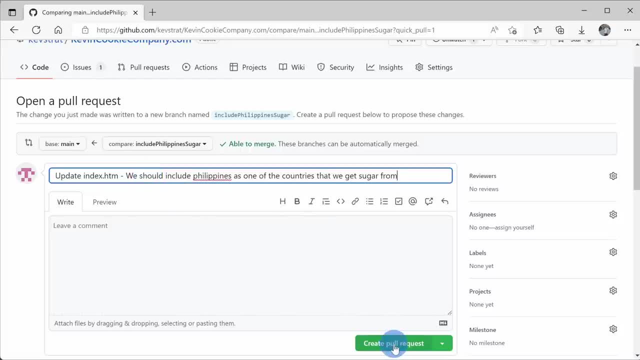 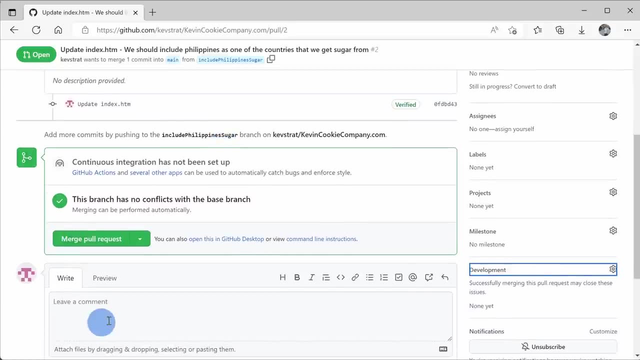 sugar from All of this now looks good, Let's click on create pull request. This has now successfully created a pull request, so we could go through and have a discussion about the merits of this change, and if everything looks good, we can then merge the pull request. 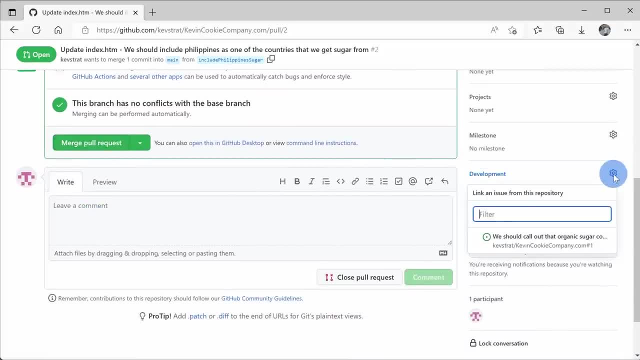 Over on the right-hand side there's a section called development, and when I click on this settings gear, I can tie this change or this pull request back to the original issue. So here's the issue that I called out, where we missed calling out the Philippines. 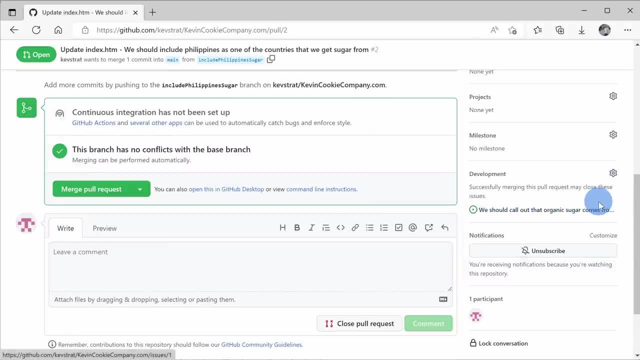 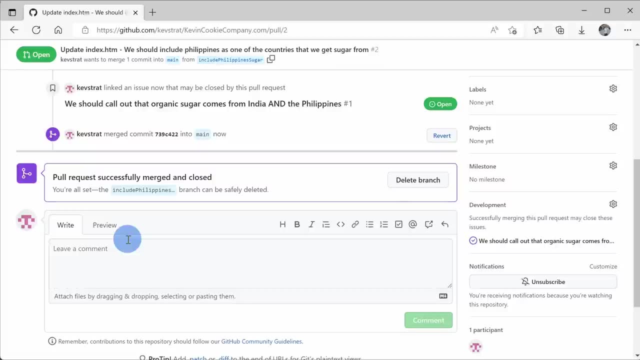 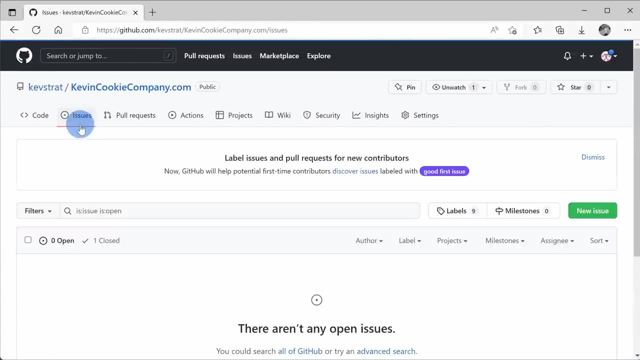 I'll select that and this is now tied back to that issue. Now, if I merge this pull request here, I'll confirm the merge. Not only will it merge this back into main, but it'll also close out the corresponding issue. Let's go up to the top of the page and click into issues. 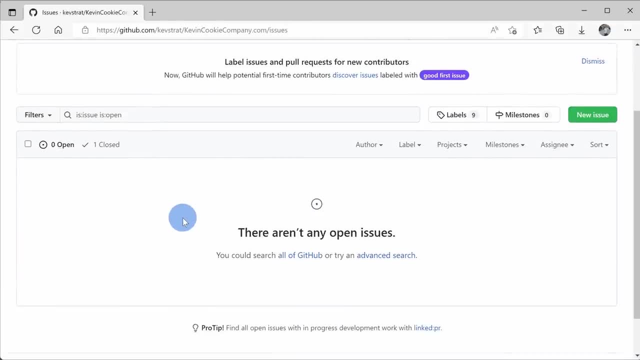 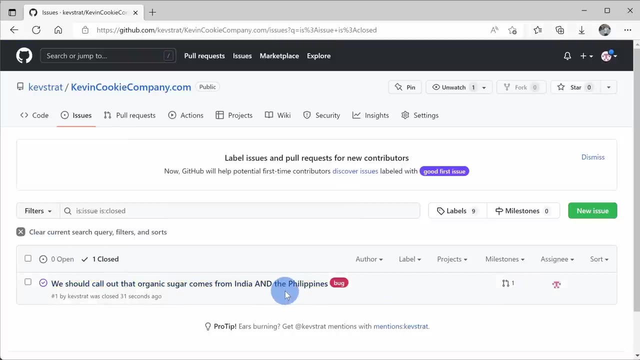 and here you'll see, because I accepted that pull request or that change, it has automatically closed that open issue Here. if I click into closed here, I could review that bug that came in and look at that. We're getting work done. That one is all done. 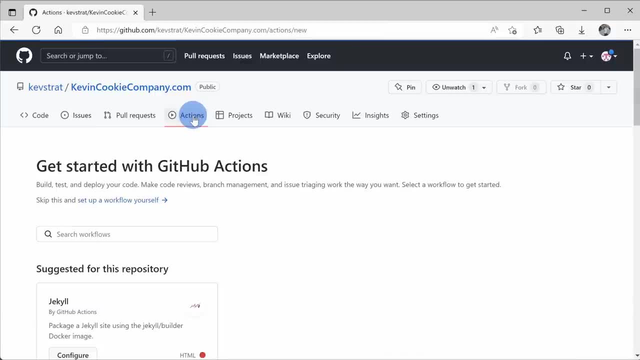 Up at the very top, there are a few more tabs. There's one called actions, and this is where you can run different tests. You could basically write programs to manage your repository. There is another tab called projects, and this is basically a project management view, where 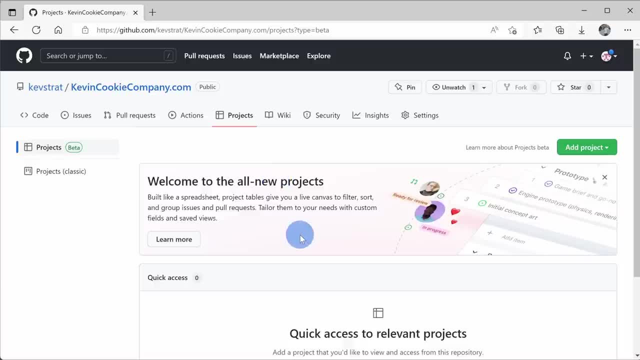 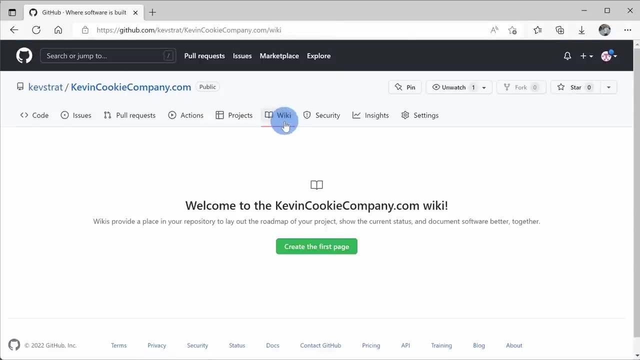 you can view all of your issues, view all your pull requests. you can filter the different views. it makes it really easy to manage your project. There is another tab called wiki, and this is where you can document your code. It's like Wikipedia, but for your project. 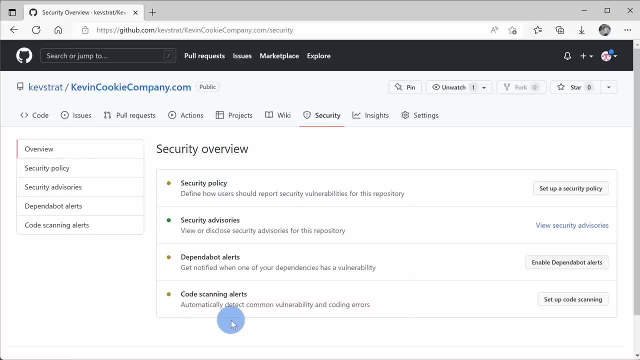 There's another tab called security, and this is where you could manage all of your different policies. You can define what should happen when, let's say, a vulnerability is discovered. You could also set up scanning, if that's what you want. There's another tab called insights. 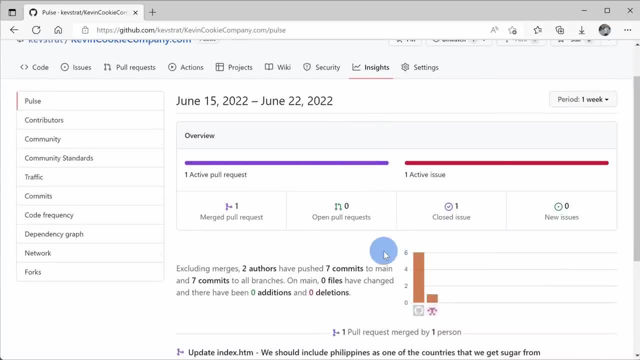 and this is where you can see well who's contributing to your project. What does the traffic look like? How long does it take for you to log in and check for anything? And there are a couple of options. There are a couple of options where you can log in and check for anything. There's. 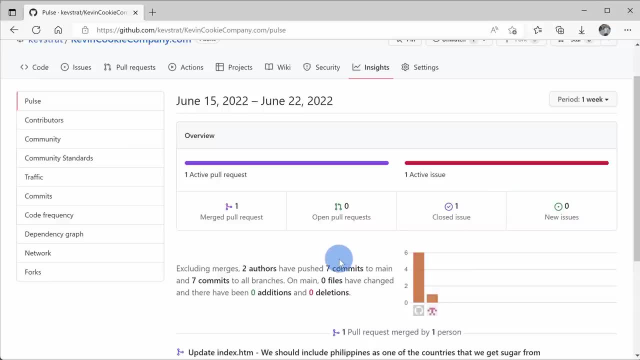 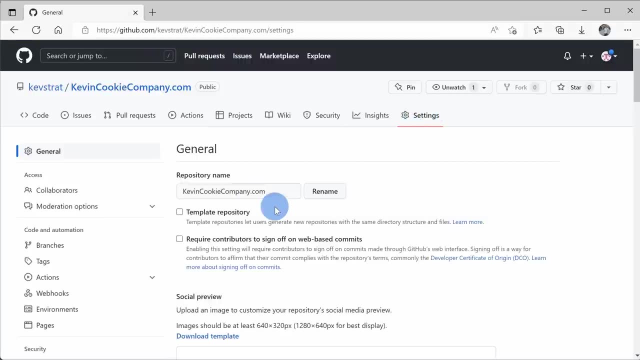 many issues have been closed, How many commits have there been, How many people are contributing? You can view all of that right here. And lastly, there's another tab called Settings, and this is where you can configure various settings related to your project. 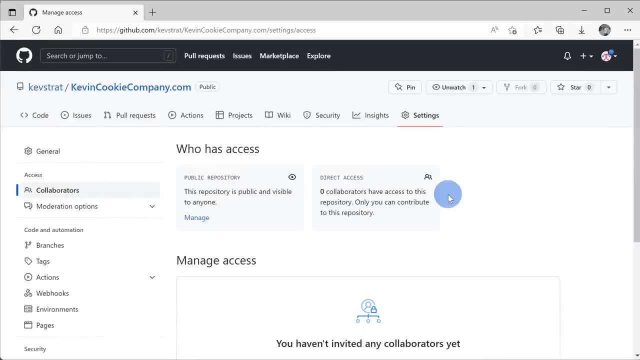 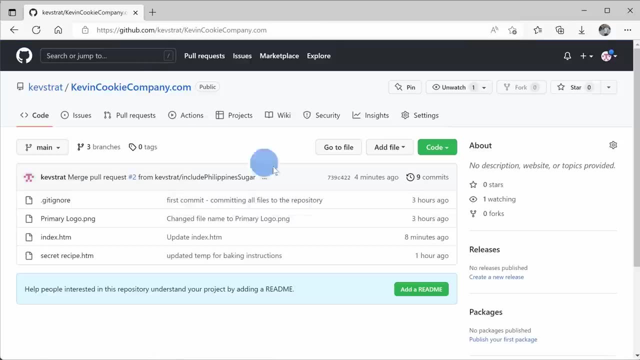 Over on the left-hand side. if you click on Collaborators, here's where you can add additional people to work with you on your project. Let's go back to the main repository view And over on the right-hand side we can also create a release. Now this is v1 of our website. Let's click here on Create. 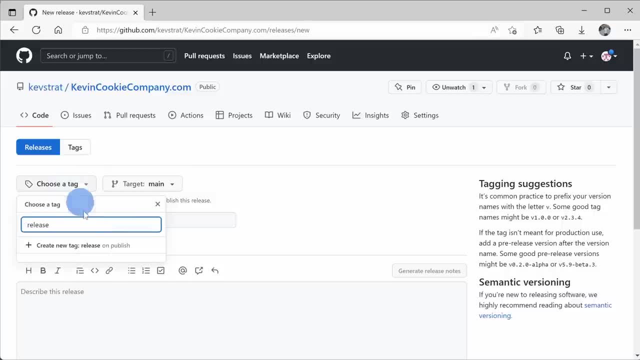 And here I can choose a tag: Why don't we call this Release? And here I'll select that, And here I can give it a release title. I'll title it v1.0.0.. This is just the first iteration. 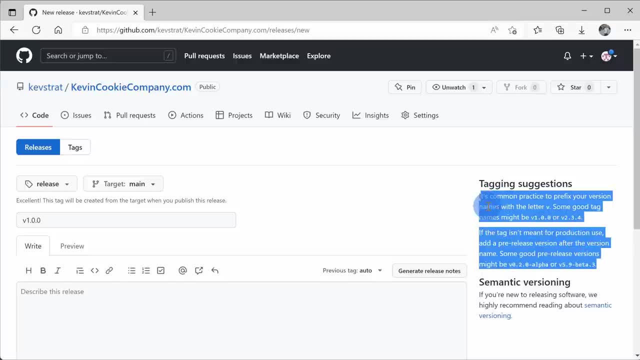 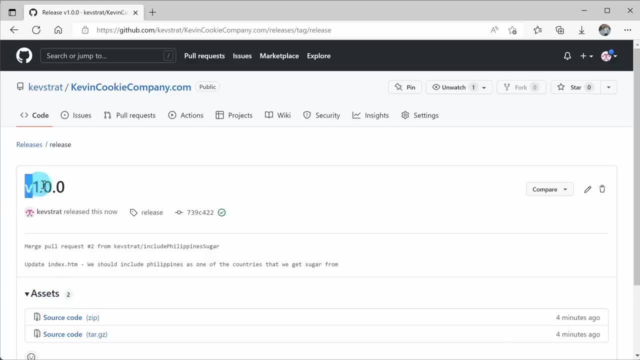 Over on the right-hand side you can see some suggestions for how you should name your release. Now this all looks pretty good. Let's click on Publish Release And look at this. We now have v1 available And here anyone can now come in and they could download the source code for.